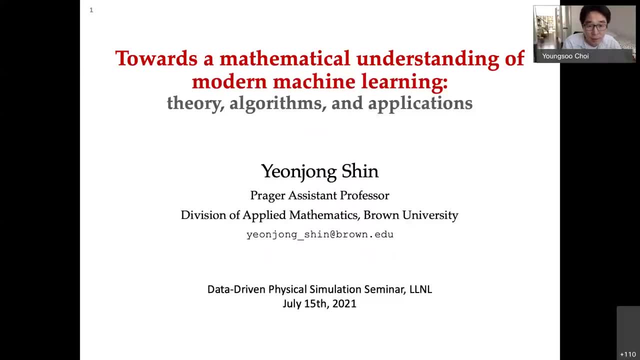 Okay, welcome everyone to the DDPS seminar. Before we introduce our invited speaker, let's go over some rules and logistics. First of all, please mute yourself during the talk unless you have questions. If you do have questions, you are welcome to unmute and ask. 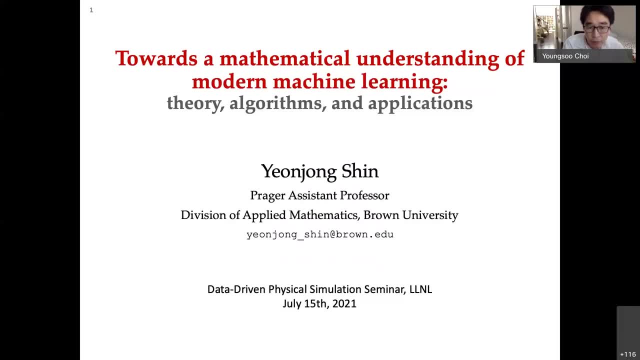 Otherwise, please use chat room to post your questions so that we can address them in Q&A session At the end. Second, today's DDPS seminar is open to the external audiences. Therefore, no classified discussion is allowed, So please watch out. 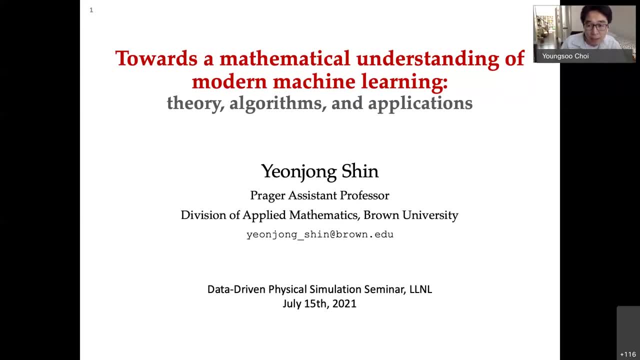 Finally, the talk today will be recorded and uploaded in our YouTube channel. That's about it. Now let me introduce our speaker today. It is an honor to host Yeonjung Shin, who is a Prager Assistant Professor at the Division of Applied Mathematics, Brown University. 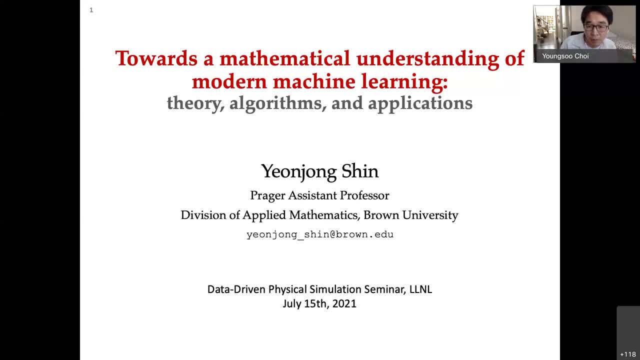 It's well known that it's a home of the Physics Informed Neural Network, which is the most popular machine learning based physics solver these days. He completed his PhD in mathematics at the Ohio State University in 2018, advised by Professor Dongbin Siu. 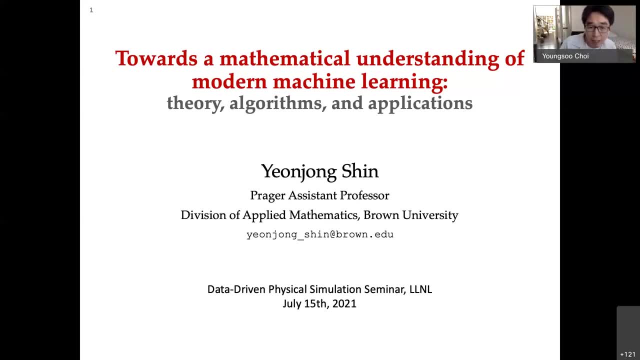 His research interests lie in mathematics of machine learning, scientific computing, approximation theory and uncertainty quantification. Today, Yeonjung will talk about mathematical understanding of modern machine learning in theory, algorithms and applications, which is very interesting topic. So please enjoy and expect a wonderful talk. 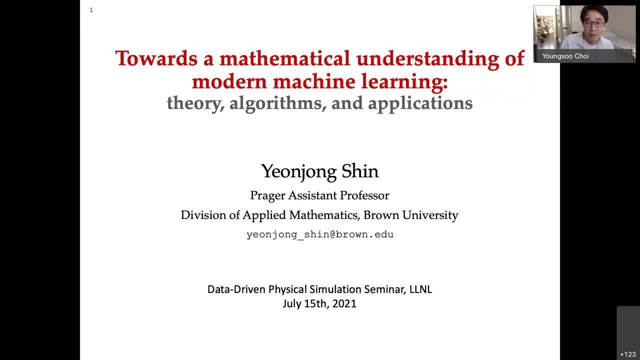 Now, without further ado, let me pass the baton to Yeonjung By asking one random question. as usual, today's random question is: what is your favorite thing to do other than research? Oh, I have one peculiar thing to do: watching YouTube videos twice faster than normal speed. 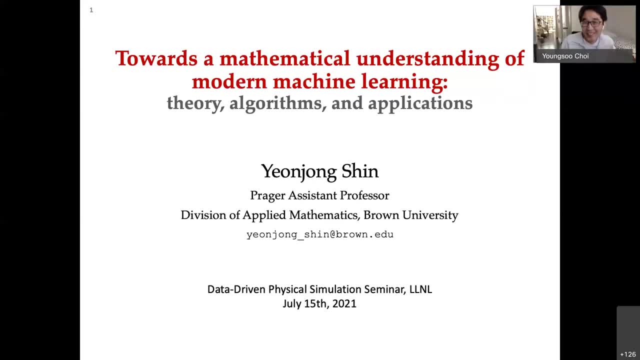 Okay, To save your time. Yes, Okay, wow And watch as many as possible. Okay, Just to see the materials quickly. Oh, wow, That is a skill. Okay, It's all yours, Yeonjung Yeah. 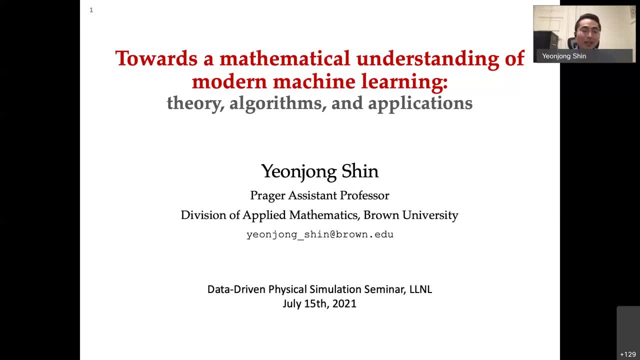 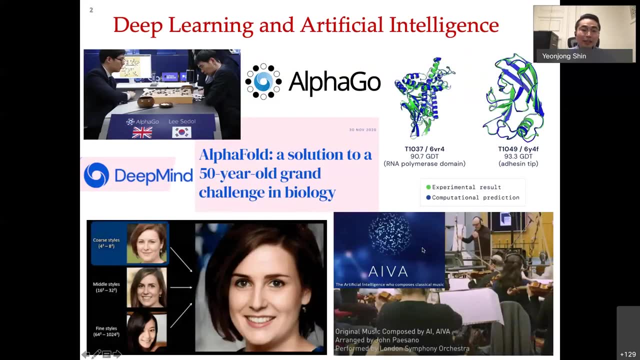 Thank you so much for the invitation. Yeon-su. Today I'm going to talk about some of my works on machine learning. Machine learning based AI technologies have revolutionized both industry and academia. It's not a big surprise to nowadays to see a news article that AI techniques can do wonder. 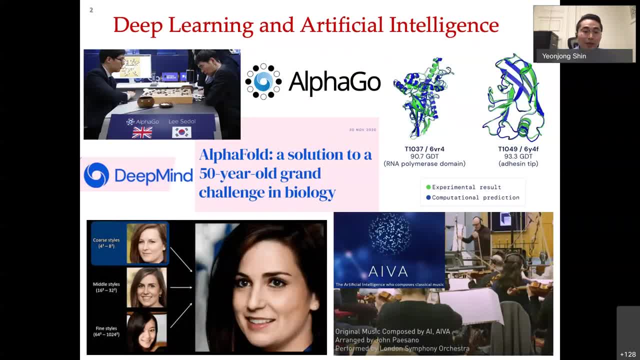 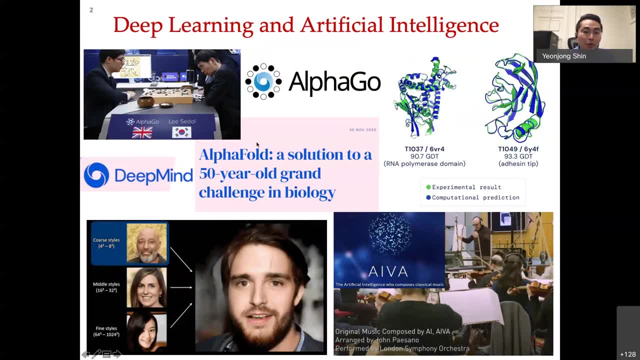 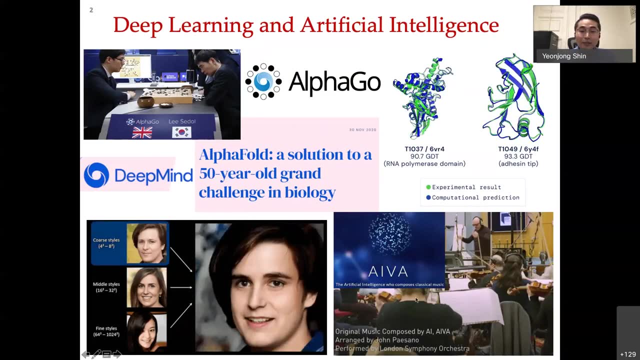 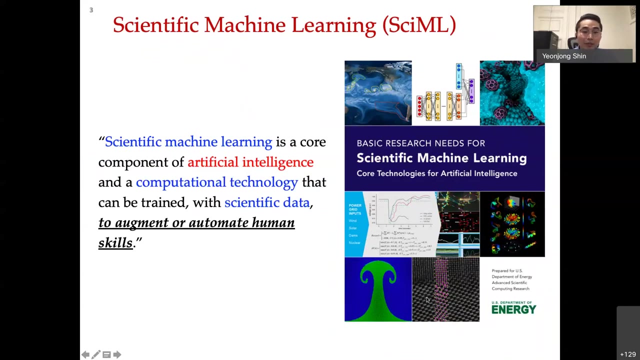 wonder it has achieved a tremendous success on many challenging applications. here i listed some of the famous examples, starting from alpha go, alpha fold and some image generations, and even ai composes classical music. and more recently these machine learning techniques have been applied to solve scientific problem. so this is the one line i borrowed from goe document. 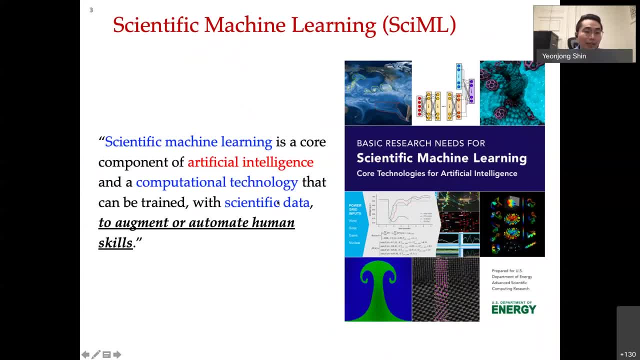 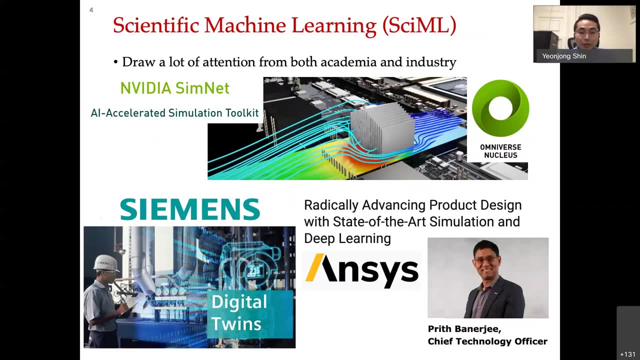 the scientific machine learning is a core component of ai and computation technology that can be trained with the scientific data to automate as human skills, and many companies also have huge interest in this field. so here i showed a couple of examples. nvidia: they use machine learning model, what they called simnet, to develop the next generation gpu. 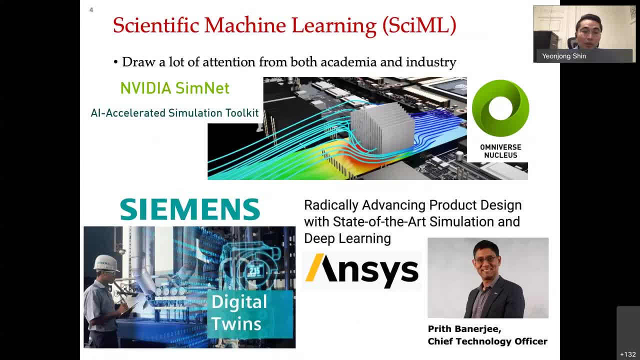 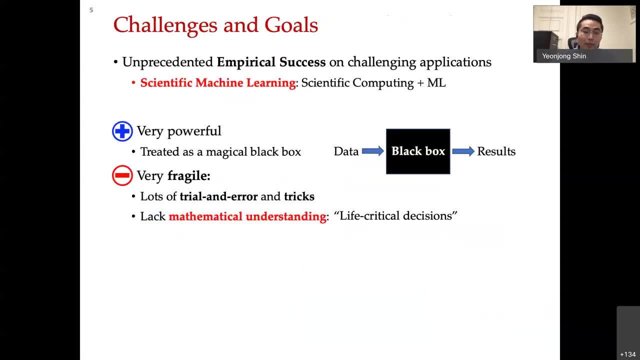 and their core technique is called physics informed neural network, which i will introduce in a moment, and also z-mans also interested in using it in their digital tool, digital twin models and also- and this is also employed- those techniques. machine learning is very powerful, as demonstrated. some people even call it as a magical black box and put whatever data they have. 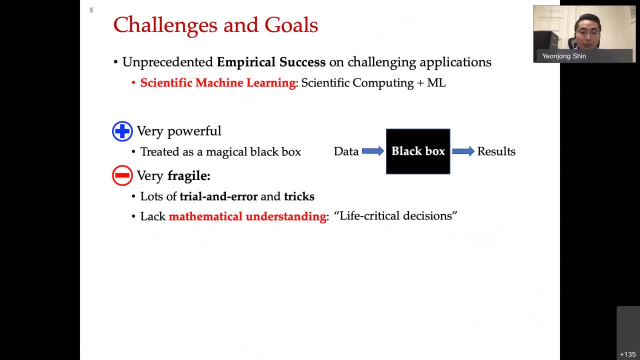 into machine learning algorithms and expect to get some great reject. however, this is not true. the theory of this success involves lots of trial and error and many tricks, and at the moment, it's safe to say that we lack basic mathematical understanding of machine learning, when it, when and 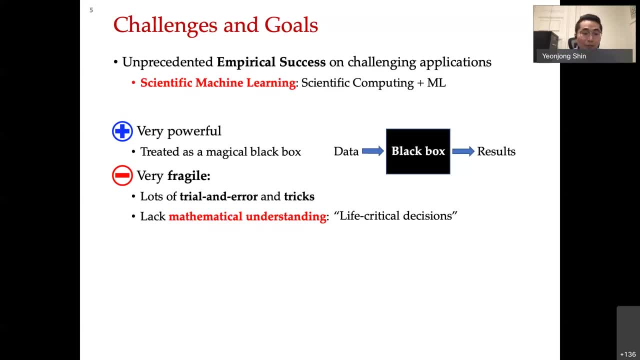 why it works. this is very important as machine learning is getting applied to make life critical decisions, such as autonomous vehicle. the general goal, says i'm an applied and computational mathematician, is to provide mathematical guarantees and, based on that, to develop fast, robust and reliable numerical method and algorithms for machine learning. then why didn't learning so successful? so what i view. 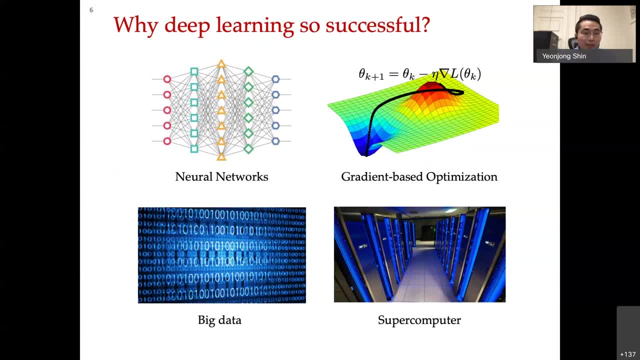 is. there are four components that leads this tremendous success. one is the modeling, which is a neural network and techniques that can train those model, which is typically done by gradient based optimization, and along with the big picture data and powerful computing power, then combining all these together, we achieve some great success. 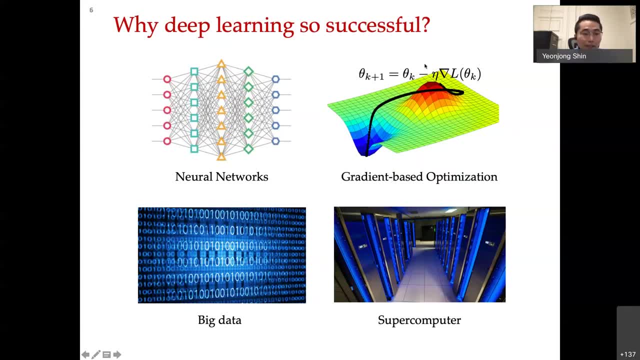 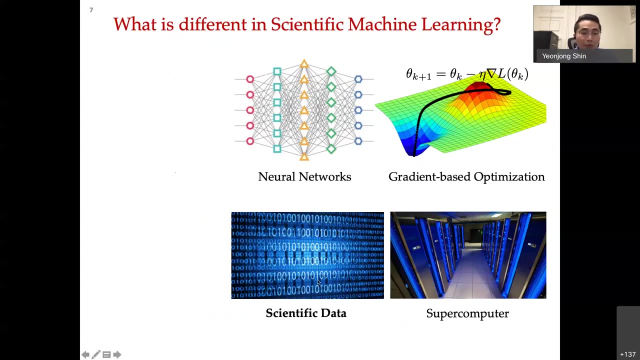 and, as a mathematician personally, i'm more interested in these two perspective neural network and the gradient based optimization. so this is a typically the what is different- different in scientific machine learning. what has been changed is the our data now become scientific data, and on the top of this we have 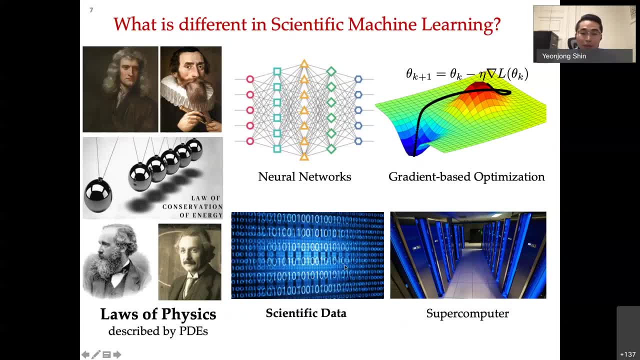 laws of physics, physical laws, are the conclusions based on long-year scientific observations and experiments. so the goal is we want to incorporate those laws of physics into the neural network, and physics informed neural network is one of them to trying to do that. the rest of this talk will be 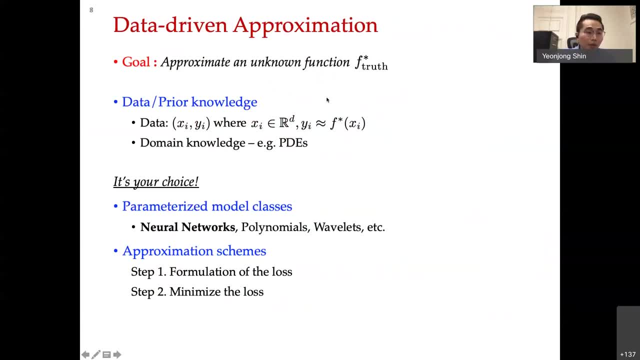 themed by the data-driven approximation. so the goal is to approximate a non-target function. f star reputation is prone to voltage gain in vez this. Sometimes Hieroglyphics also lead to unambiguousuddinging importance in scary things. One is the parameterized model classes. So in this talk I will focus on neural network. 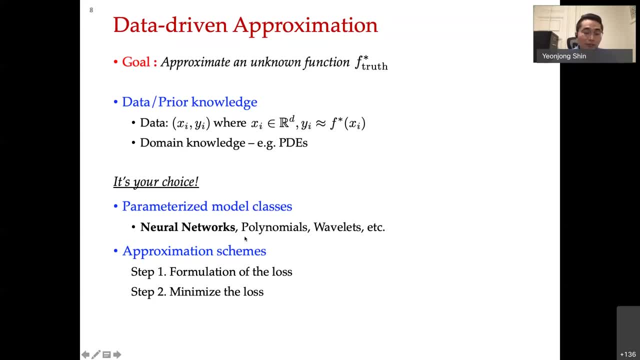 but classically we were a numerical analyst, were using polynomials or wavelengths, And once the parameterized model classes were chosen, the next thing is to decide approximation schemes. Approximation schemes can be decomposed into the two steps. The first step is the formulation of the loss and the second step is the minimized the loss. 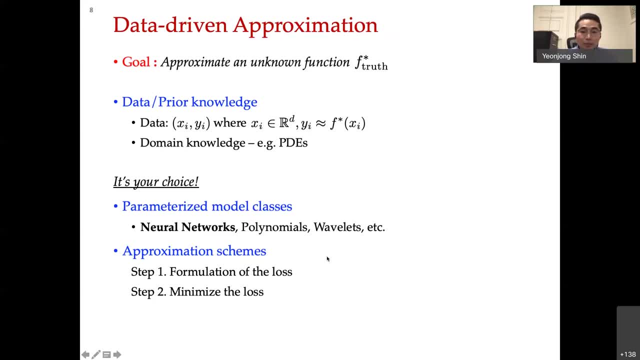 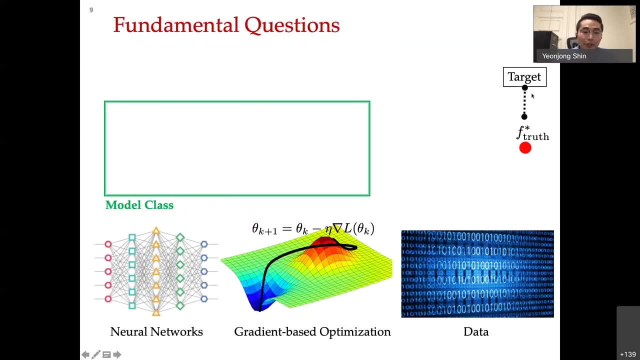 Then this actually creates the multiple fundamental questions which I will illustrate in this slide. Suppose f: star is our target function. we wish to approximate and to do this we choose a model class In this talk. this model class will be neural network. Then let's say h: hat is the best model. 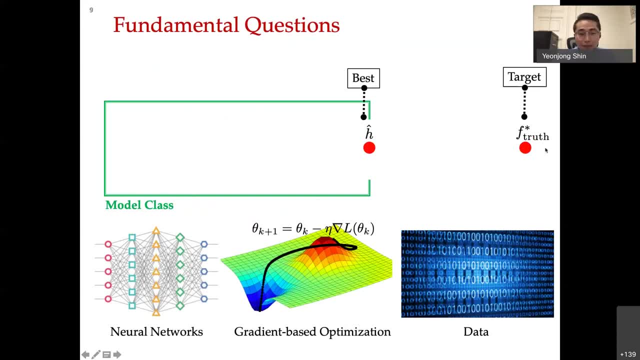 belongs to the previous model. We will go through this model class and see how the model to be approached to this model class to approximate this f star. Then study of these two difference and this error is called approximation error. and study of this error belongs. 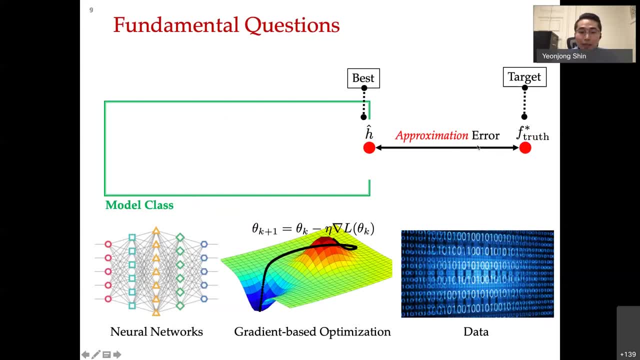 to the classical approximation theory. In this error data doesn't play any role. So this error is completely determined by our target function and your choice of the model class. So there's no data placing a role in this error. And now data comes in, we define a loss function. 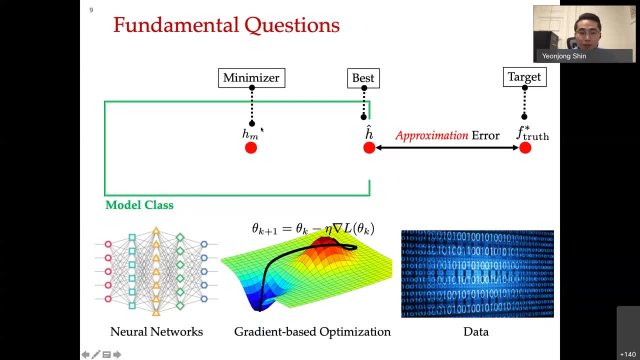 Then let's say HM is our minimizer of the loss function. Here small m is denoted by the number of the data. Then the difference between this minimizer and the best function is called estimation error. This error comes from the finiteness of our data. 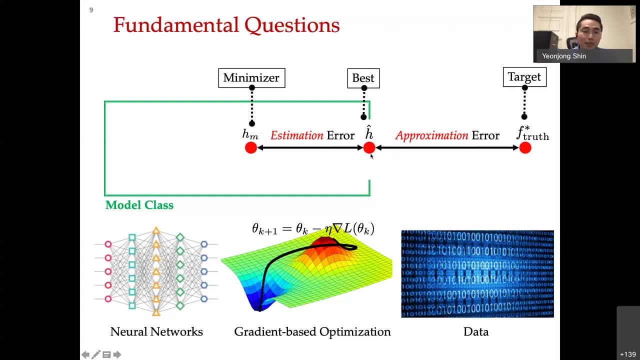 If we were to have infinitely many number of data, then this error will be zero. Then, combining these two error together, we call it generalization error. So in some sense the understanding generalization error is the realm of some theoretical work. But what we see in practice after training? 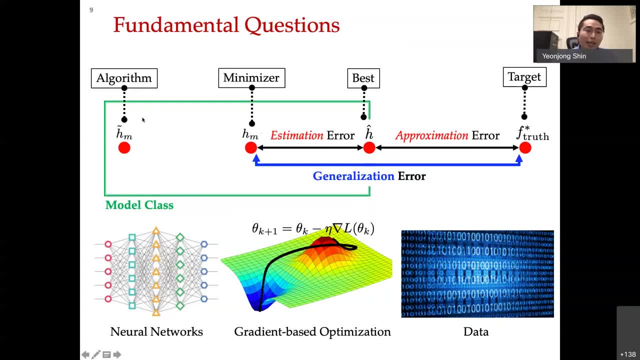 on the gradient descent algorithm, what we get is H-tilde. So this is the outcome of our algorithm. Then the difference between these two is called optimization error. So in this talk I will going to talk about gets past, om the point's al for hochchoice. so in this talk I will going to talk about 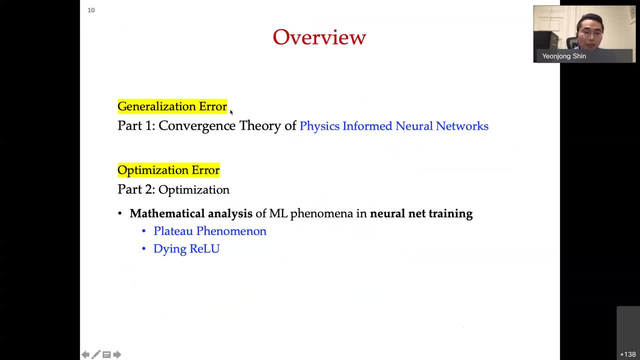 the both. So this is the outcome of our algorithm. then the difference between this two is called optimization error. So in this talk I will going to talk about- So first part, I will talk about the generalization error in terms of the physics-informed neural. 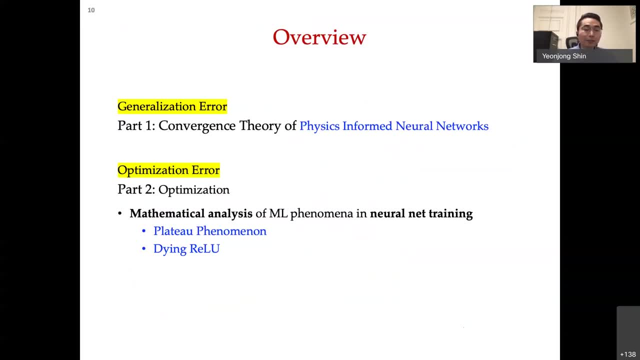 network. And the second part I will focus on optimization, especially mathematical analysis, of some machine learning phenomena in trained neural net, the Philatel phenomena and the dying-ray loop, Since all of those topics involved in neural network. so let me first just go over what 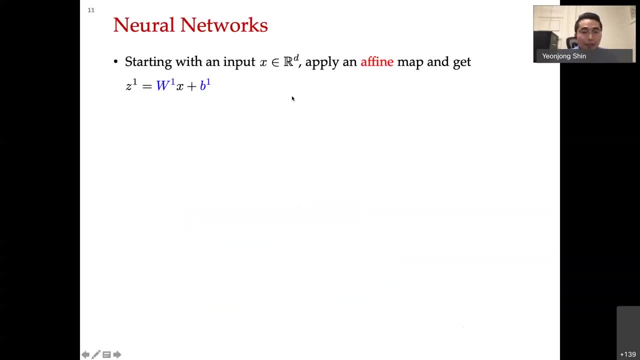 is neural network. So, starting with the input, X lies in D-dimensional space. we apply an affine map to get Z1.. Here W1 is a matrix, B1 is a vector and W1 is called a weight matrix and B1 is called. 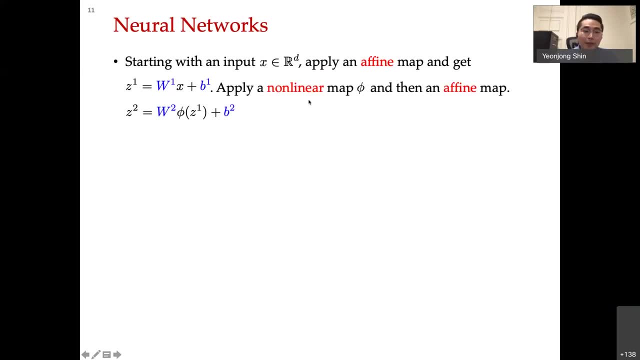 bias vector. And then we apply a nonlinear map, phi, and then again another affine map to get Z2. And then we repeat this procedure until we get ZL. Then the map phi is a vector. The mapping from X to ZL is called L-layer neural network. 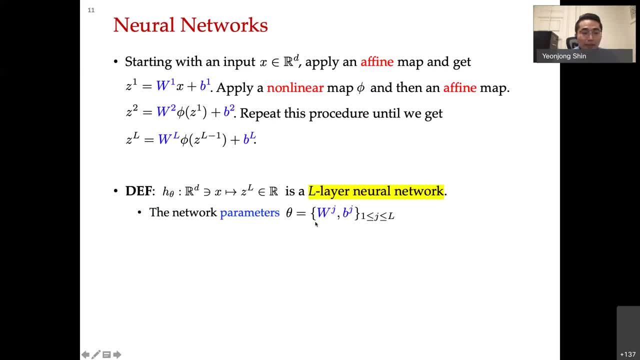 And the collection of those weight matrices and the bias vector is called network parameters and this is something we need to learn. And the network architecture is just a collection of the size of the weight matrices. So, for example, W1 is the matrix of size N by D. 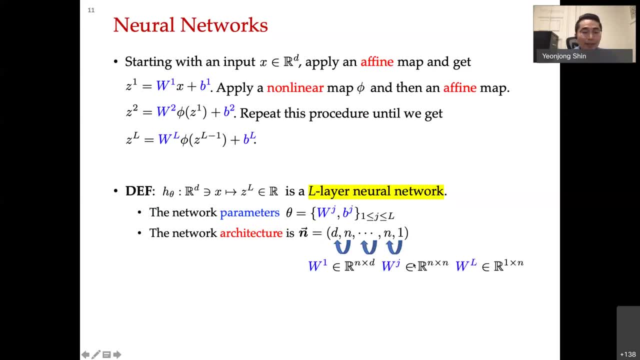 And intermediate layer is the weight matrix, Intermediate layer is the N by N and the last layer is the one by N. Here I assume the output is just a real valued function And typically L is called the depth of the network. small n is the width of the network. 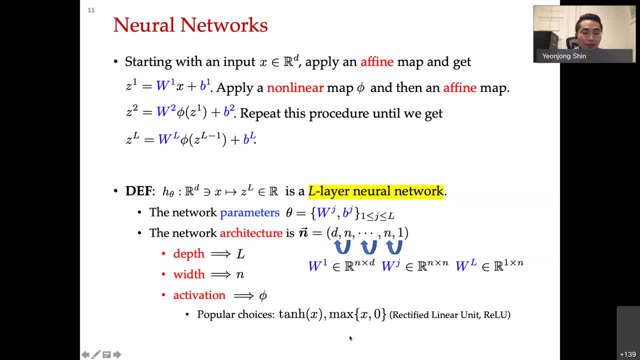 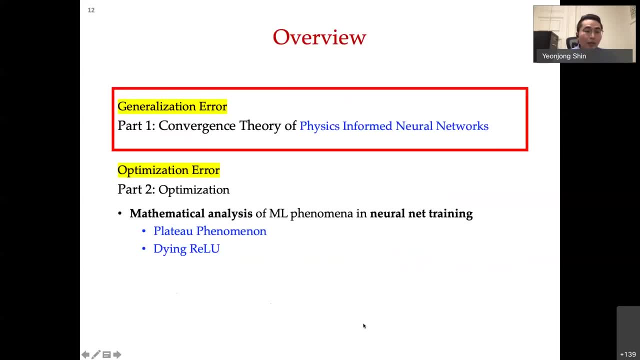 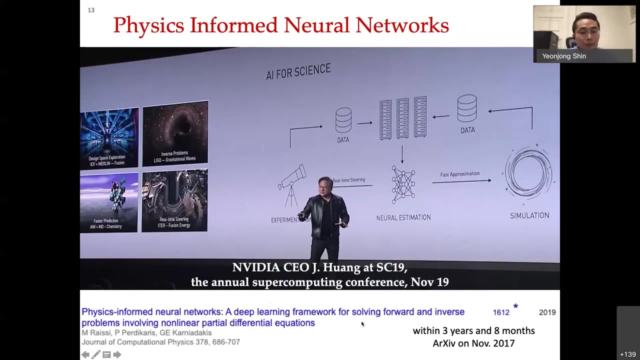 and phi is called activation function, Some popular choices: the hyperbolic tonnage and the ReLU function, which is just a max function. Now, with that, let me talk about the comparison, Okay, Okay, Let's talk about the convergence theory of a physics-informed neural network. 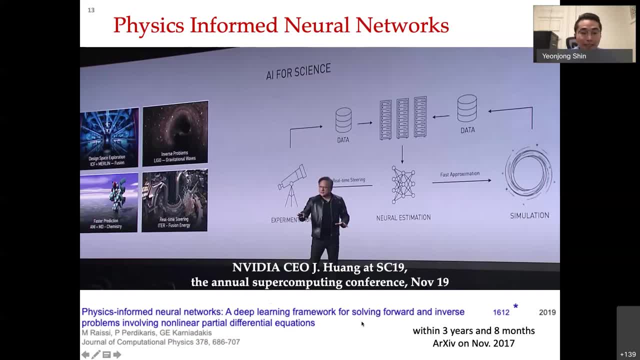 Physics-informed neural network is a deep learning framework for solving PDE. This was first appeared on the archive in November 2017, and merely within three years and eight months, it already cited more than 1,600 times, And PIN also has appears on media multiple times, but here I show the first time I saw. 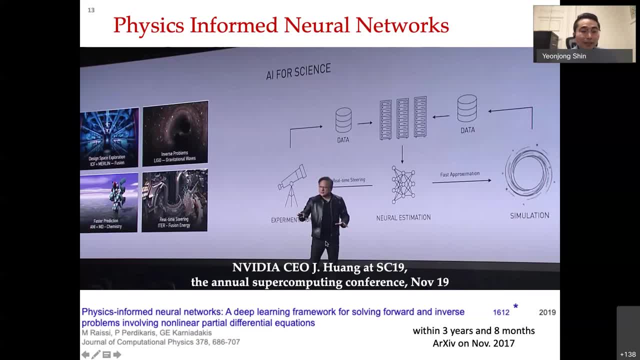 PIN in the media. So NVIDIA CEO Jensen Huang addressing AI for science in the supercomputing seminar in 19, and he's mentioning PIN. The principle is the same as before trying to embed the physics equation into the neural network. 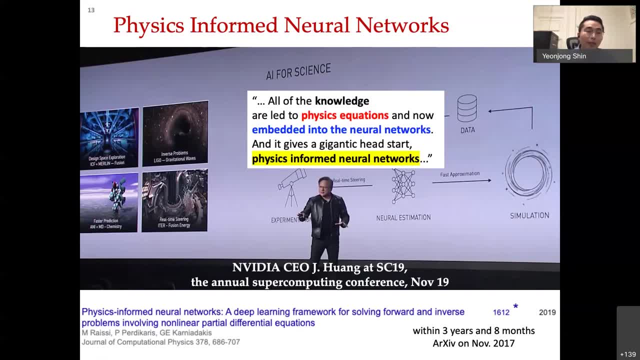 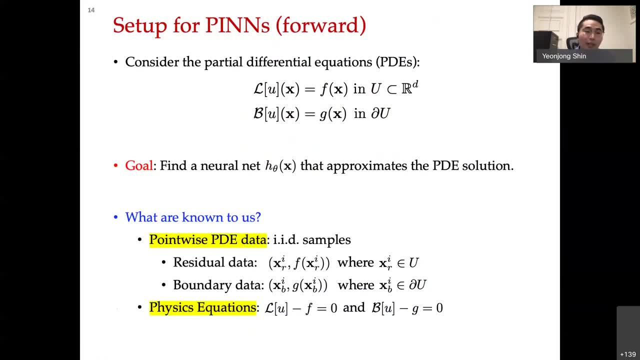 And one way of doing it is the PIN. The setup for the PIN goes follow, So I will focus in on the for the problem, although PIN can be applied for both way. but for theoretical analysis, I will focus in on the for the problem. 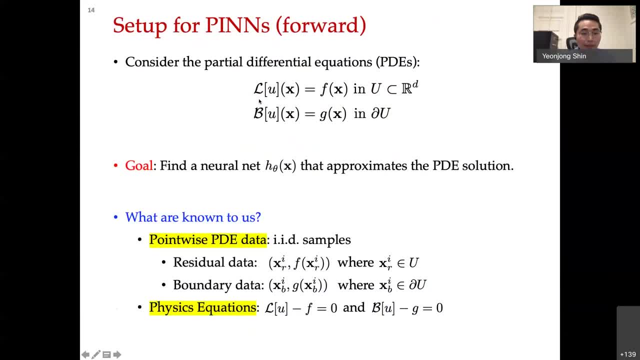 So we consider the following PDE Here: L is the differential operator and B is a boundary operator And F and G are PDE data and U and boundary of U is just a standard, the open and bounded. Then the goal is to find a neural network that approximate the PDE solution. 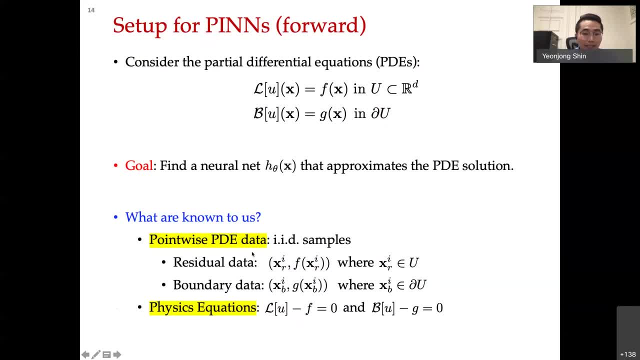 And what are known to us is the two things: One is the pointwise PDE data, Some data from the Interior and the data from boundary, And if you completely know about F and G, then this you may think of this is not a data. 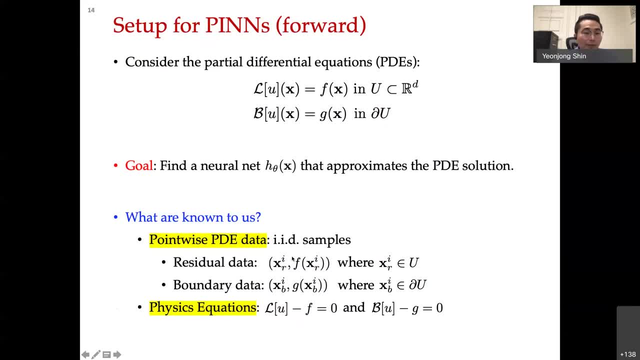 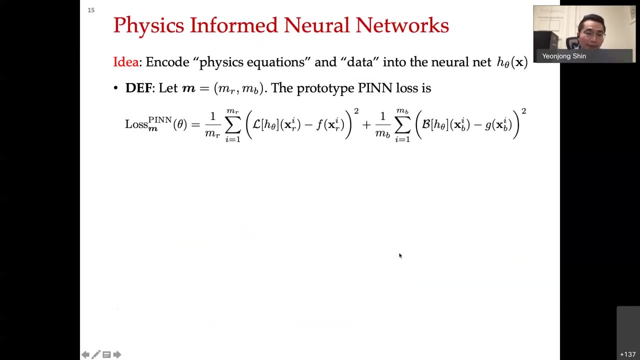 or something you can get freely. But if you don't know F and G, then you can treat this as a data And on the top of that we might know. we know the physics equation in terms of L and the B. So, as I said, the goal is to encode the physics equations and the data. 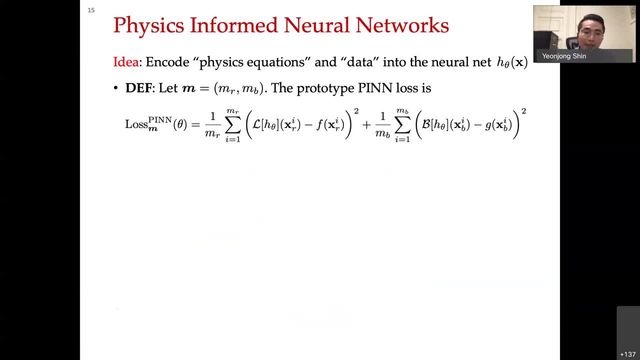 In The neural network. then how we do this for the pin. the original work proposed to do this job by minimizing the loss function. then prototype pin. loss function is defined in the following manner, composed with the two terms: One is the mean square loss of the interior part, both physics and the data. 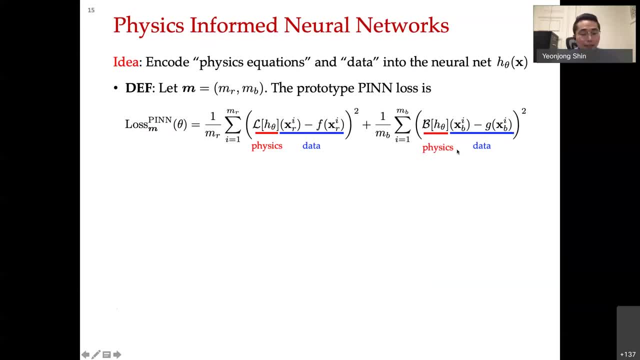 And the other term is the mean square error of the boundary physics and the data. The method Is To minimize this pin loss function And we get the minimizer, which is the network parameter. And by using this minimize the parameter back to neural network, we get a physics informed. 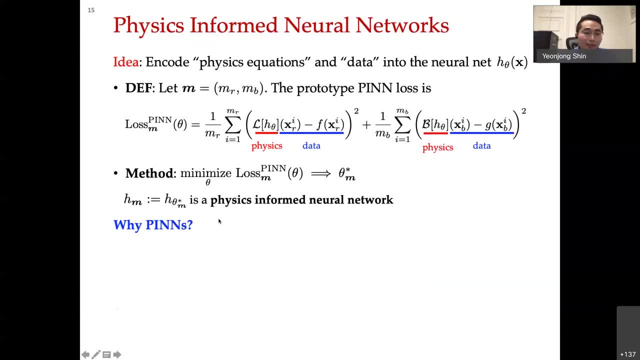 neural network. The white pins. there are multiple pros and cons for the pins, but one, one part is easy and simple to implement it. and someone, someone said- someone, also saying as a joke- that high school student can solve the Schrodinger equation using pin after spending a couple of hours. 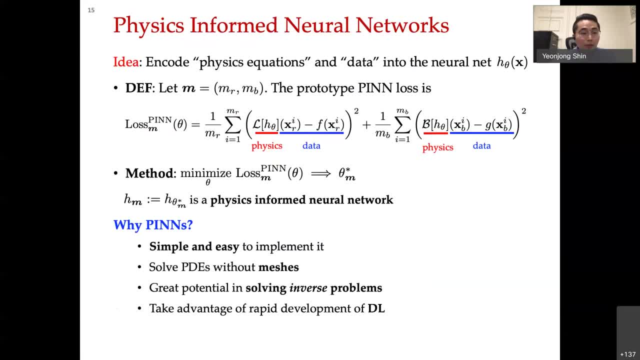 And the second one is the is one of the methods that solve the PDE without meshes and also great potential in solving inverse problem especially, and also take advantage of the rapid development of deep learning. Yet it lacks a theoretical understanding and also has some potential issues in the. 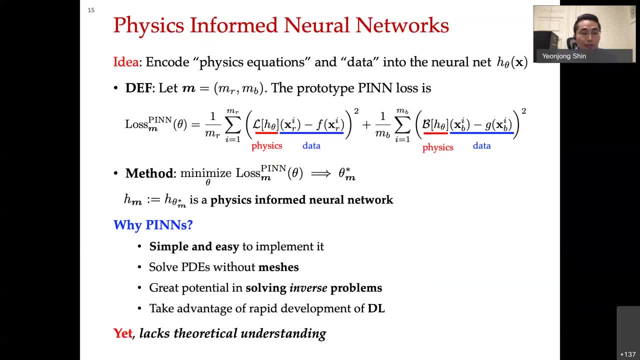 optimization procedure. But at the moment, for the first part, I will focusing on just the theoretical analysis, assuming minimizer is achieved. And one natural question one might ask is the consistency. consistency, uh, reject meaning that Here M denotes the number of the data point. 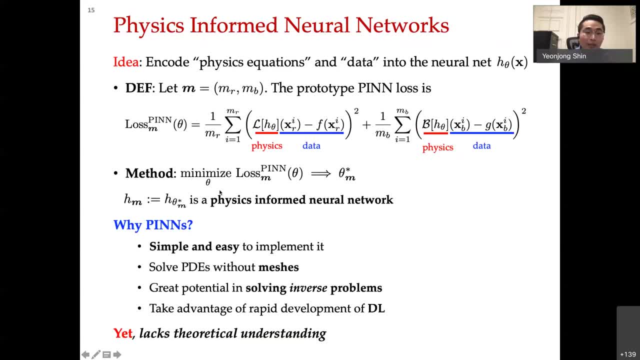 Then for fixed number of the data point, we get a neural network, physics informed neural network. Then the natural question- a natural question would be: as the number of the data point increase, we get a sequence of the physics informed neural network. Then the question is: will this sequence of physics informed in your networks converges? 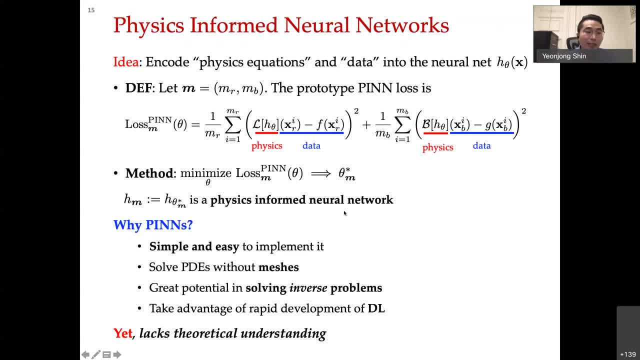 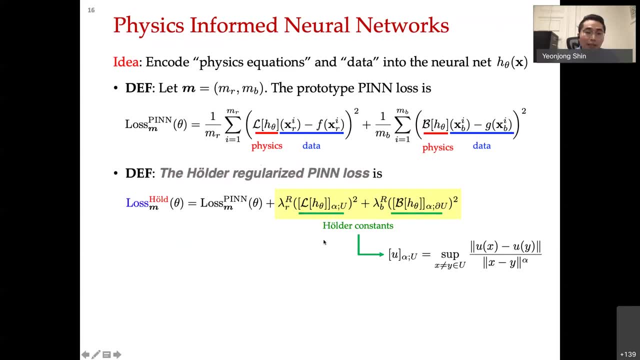 to the solution to the PDE. If it is, then we say it is the consistent. for the analysis. We proposed the called held a regularized pin loss. It is the regularized pin loss, In particular Of the held, a constant of the L of the neural network and B of the neural network. 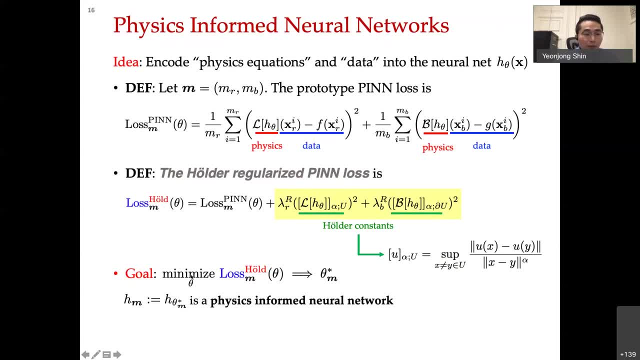 So we are going to focusing on the following problem: minimize the held, a regularized pin loss, And say that star is our uh uh optimum parameters, that we get a neural network. And as the number of data increase, we get a sequence of the neural network. 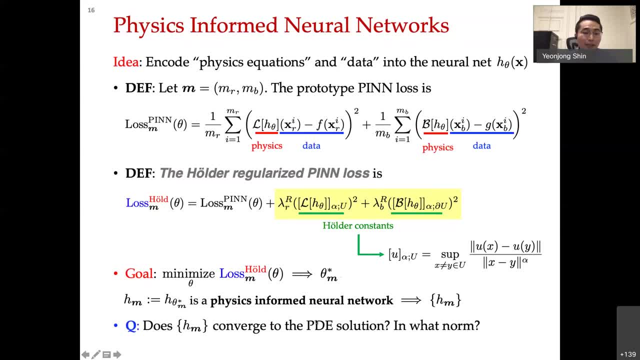 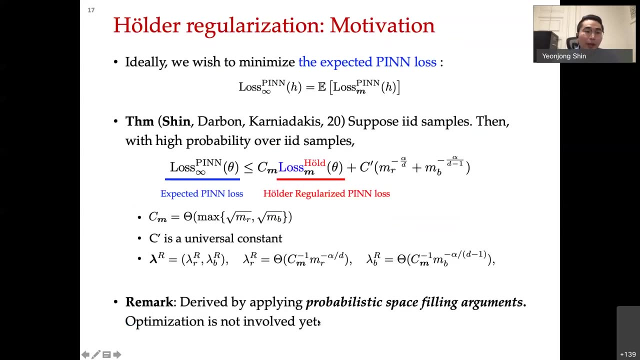 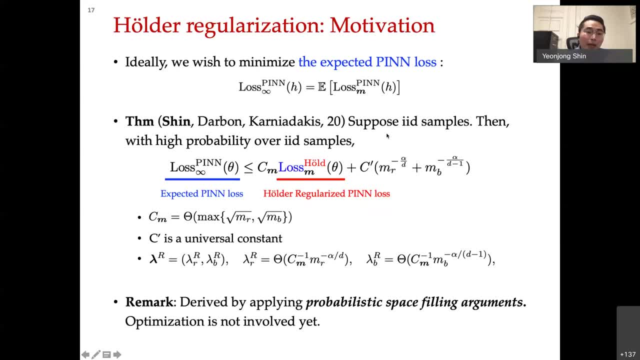 But 1 theory we prove is the following: Uh, by assuming our samples are then with high probability Expected, the pin loss can be bounded by held, the regularized pin loss. And uh, these other term actually goes to 0 as the number of the data increase. 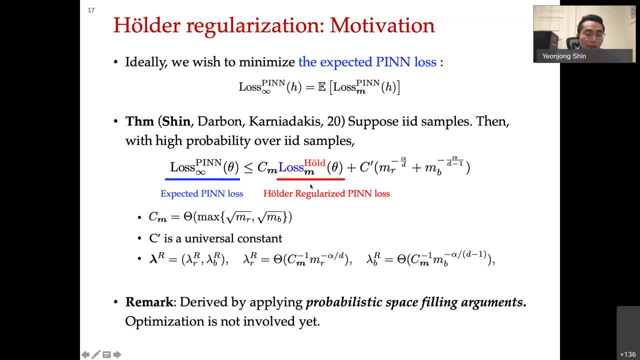 And this uh, this uh suggest: 1. Way of controlling expected the pin loss in a nice manner And in this upper bound. actually, we did not apply any optimization procedure yet, So this is purely obtained by applying probabilistic space of filling argument. 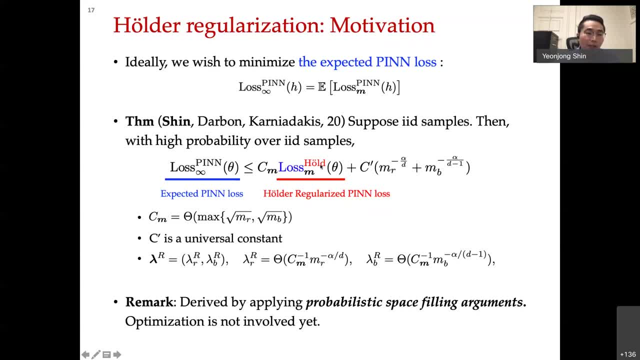 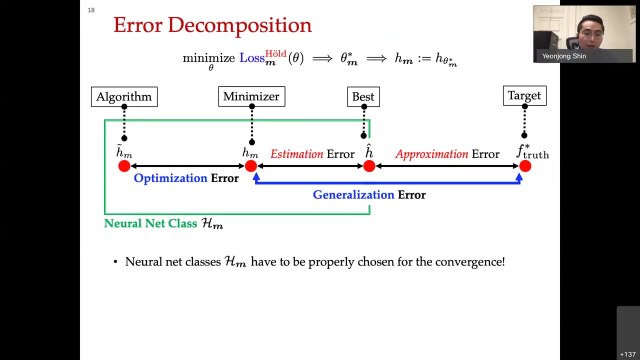 So, by applying the optimization, By reducing this well, the regularized loss is sufficiently decay fast that we can expect to get some convergence. So in order to guarantee the convergence, we need to uh Impose some proper conditions on the neural network class. 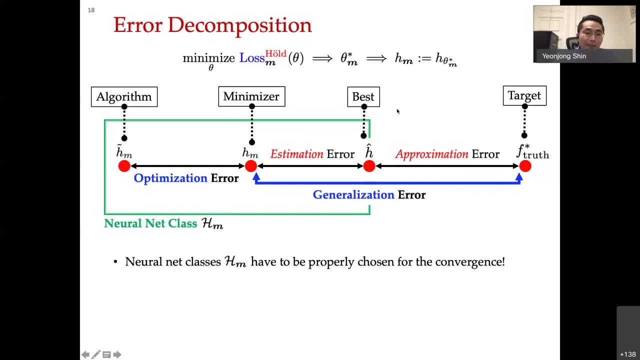 Because what we get is this, which is minimizer, And in order for the convergence, we need to uh, Sort of like guarantee that this generalization error goes to 0. Which means that approximation error has to go to 0, which means that your network class. 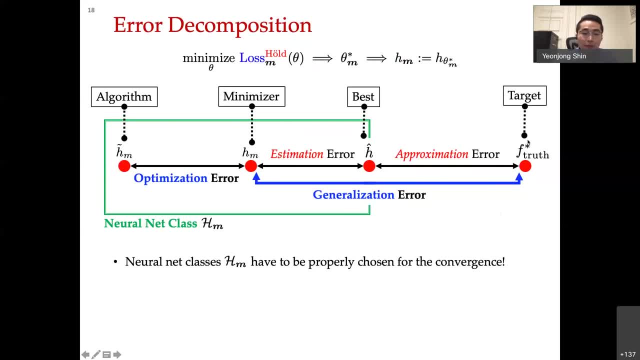 Should it be sufficiently large enough to capture this target function. at the same time, We need to a way to control this estimation error So that we can reduce the convergence, we can uh Drive the convergence and from now on, for the ease of the notation, I will use this functional location because, uh, your network is determined by the network Convergence. 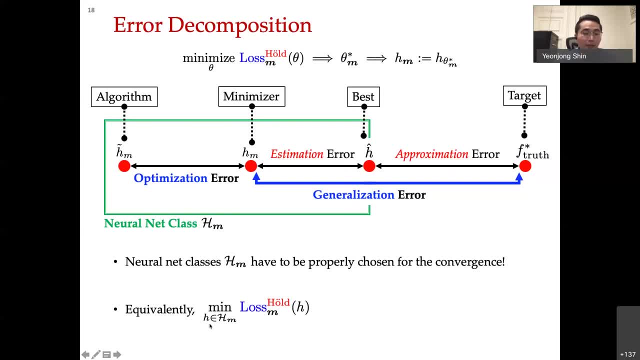 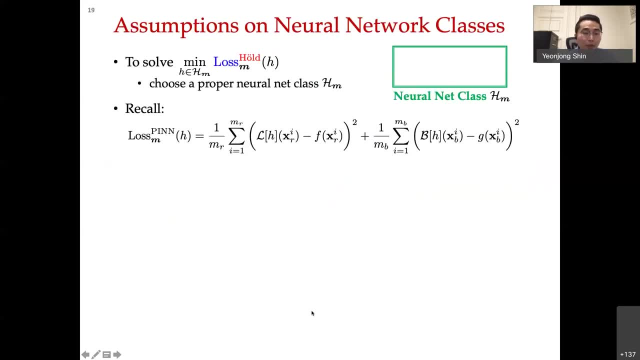 Parameter, meaning that we can choose a function in the Your network class. so I was going to use this functional location. Then there are 2 key assumptions on the for the convergence. 1 is interpolation of the data. There exists a function, the neural network, that interpolates the 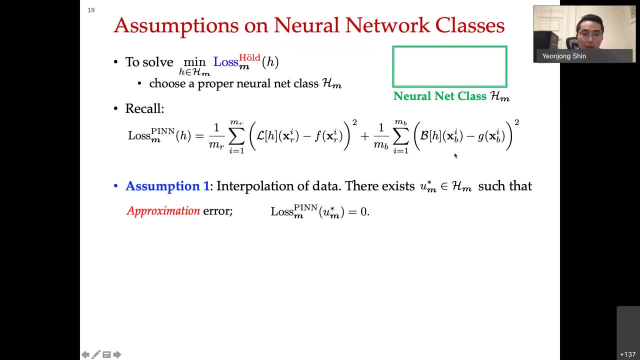 The data, which means that achieve the 0 pin loss, the prototyping loss. this assumption controls the approximation error. And the 2nd assumption is the uniform boundedness of the held a constant, And this controls the estimation error. and these 2 assumptions are essential for the proof, Although the assumption 1 can be relaxed a bit. 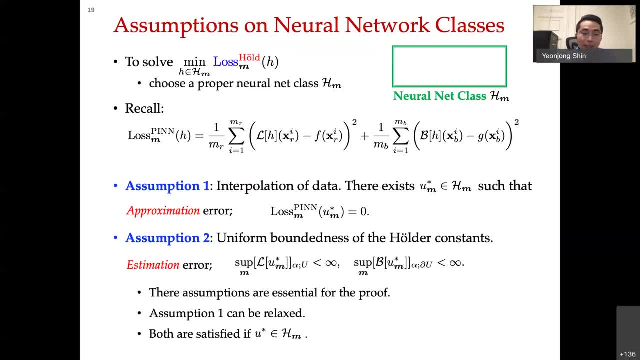 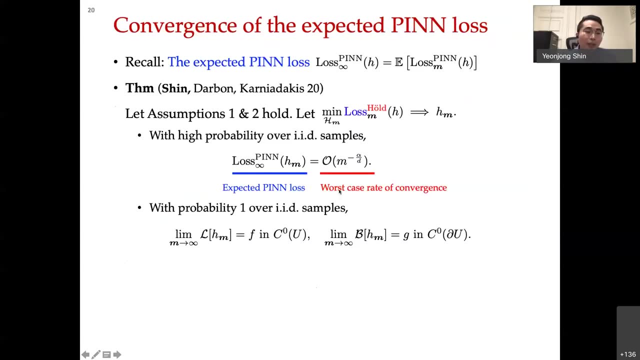 Yeah, these 2 assumptions can be both satisfied if there exists a neural network. Uh, that is exactly the solution to the. Then, with these 2 critical assumptions now we can have some Convergence. Richard, supposed to assumption 1 and 2 hold. 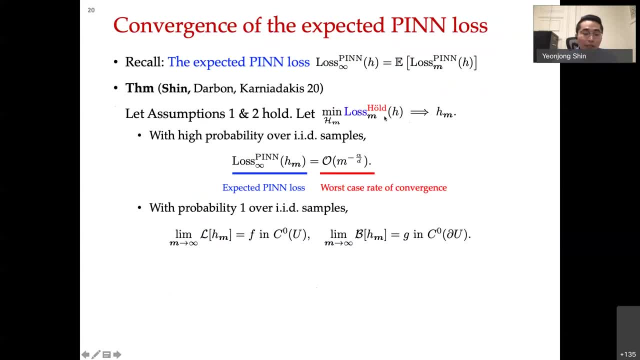 And let's say HM is the minimizer of the held a regularized loss, Then with high probability expected, the pin loss Evaluated at our minimizer actually converges to 0, with the following rates: So this is the worst case rate of conversions: 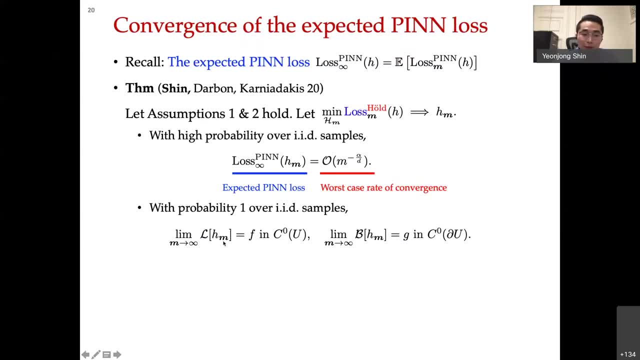 Furthermore, L of the physics informed the neural network, B of the physics, Some informed the neural network converges to the PD data uniform. So this is the great Richard, In the sense that we guess we can guarantee some sort of like convergence after applying the operators. 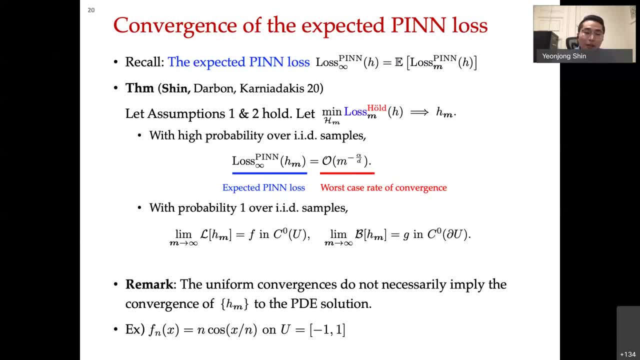 However, this uniform conversion is not strong enough to conclude the conversion to the PD. So 1 example is this: so that all the derivative converges to 0 uniformly, but function itself does not. So this is the moment we need to specify what kind of the class of the PD we are looking for. 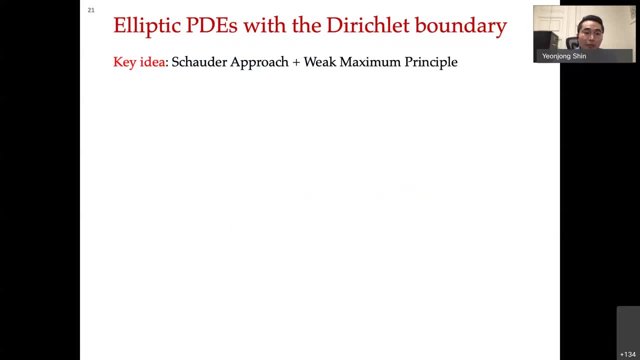 So, in that we actually borrow the shelter theory from PD and combine it with the maximum, with maximum principle, The shelter theory guarantees the, the point, wise evaluation and sufficient regularity and the uniqueness of the solution And, with maximum principle, controls the how we deviate from the boundary. 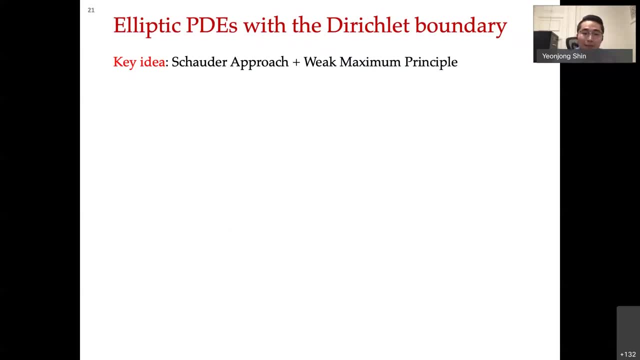 Because, unlike other PD method, pin does not enforce the boundary condition to be satisfied in the 1st place. So there must be a some uh technical tool that controls the boundary values In in some nice manner. and that is the weak maximum principle. 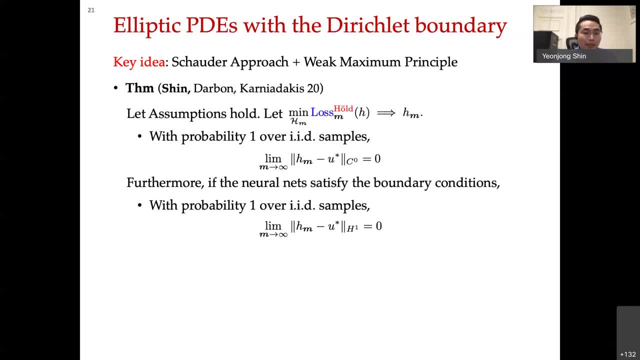 Combining all this we can now have a nice convergence theorem, Suppose the assumptions hold, conclude Involving the shoulder assumption and with maximum principle and uh 2 assumptions that I mentioned earlier and is the minimizer of the regularized loss. 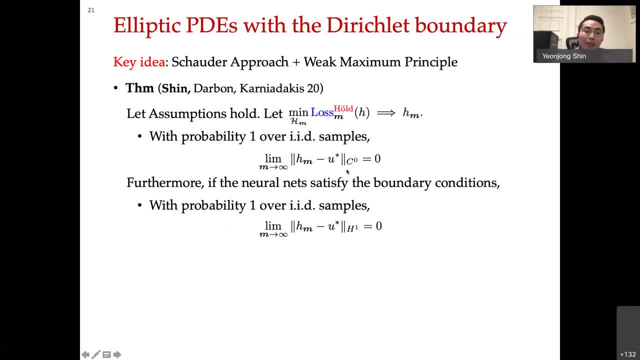 Then, with probability 1 over sample Sequence of the physics informed, the neural network converges to the solution to the PD uniformly. And furthermore, if the neural network satisfy the boundary conditions exactly, then the convergence mode to become H1.. And here are some proof idea, but let me skip it. but similar result holds for parabolic case. 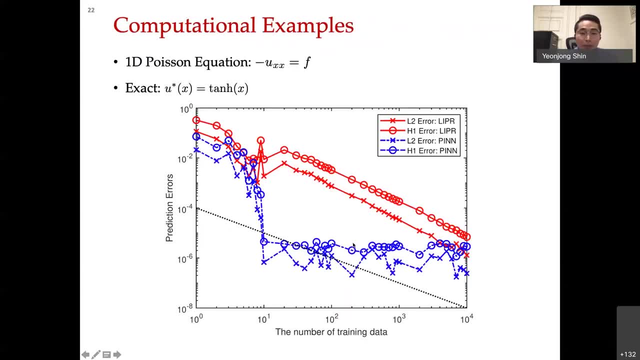 Here I show some demonstration. So the purpose of this plot is to just illustrate the convergence of pin to the PD solution. Just what I just to show you before. So here I consider the special case where uh held exponent is 1, which becomes the latest. 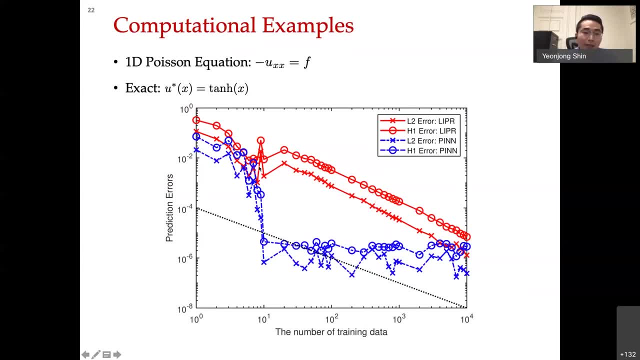 Regularization, which is shown by red, And uh standard prototyping loss, which is shown by blue curve, And here dashed line is the rate of convergence. from our theory, Then you can see that uh theoretical result is well observed by the numerical simulation as well. 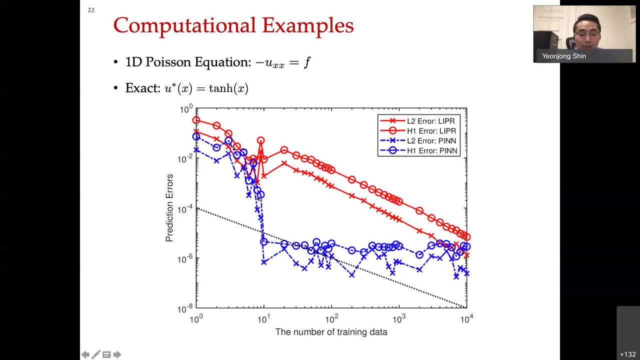 And but what? what is interesting is actually the. Without any regularization, just a standard physics informed, the neural network seems to converge exponentially fast and saturate Afterwards, Which is something we cannot guarantee from the theory. But red 1 is guaranteed by the theory and similar which are told for the. 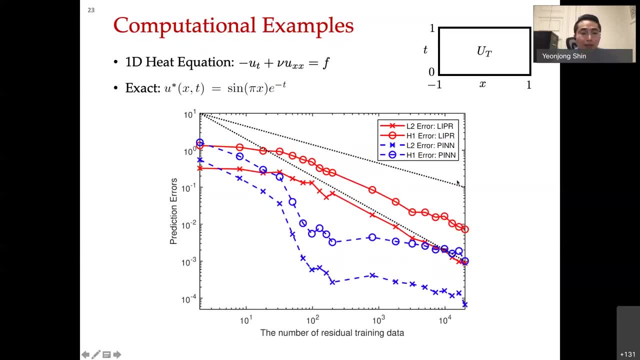 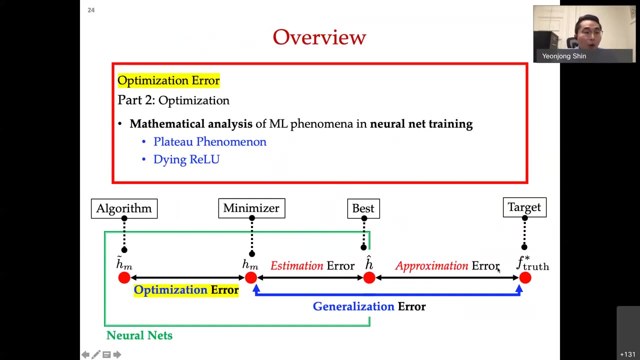 Key to equation. the upper dashed line is our theoretical line and the red 1 is our numerical simulation. And the blue 1 is the standard physics informed the neural network. Now let me move on to my 2nd topic, which is the optimization error. 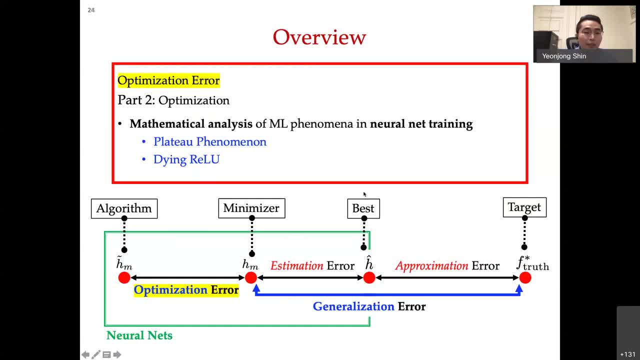 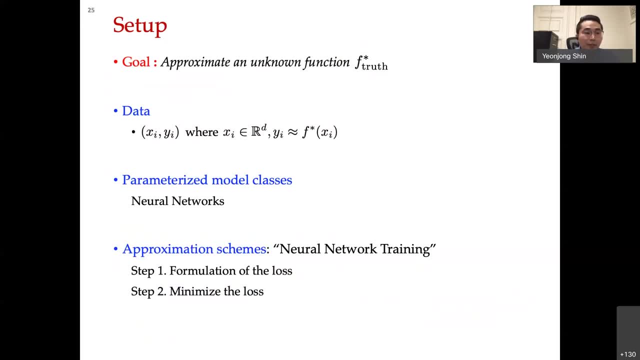 So mainly I will going to discuss the 2 thing. 1 is the flat to phenomena and the dying Ray Lou For the optimization. the setup is the following: the goal is to approximate an unknown target function and for store, And our data is just X, I and Y I data set. 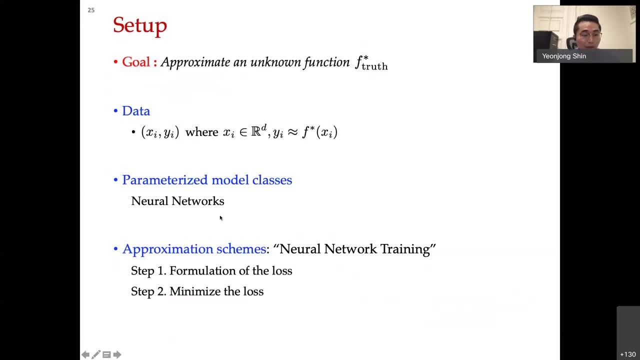 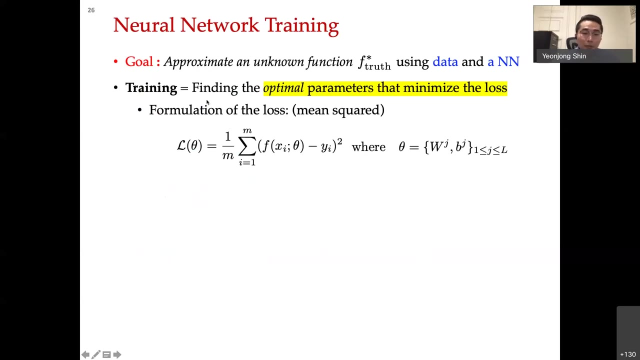 Uh, and model class is the neural network And approximation scheme is the neural network. training, which I will going to Uh Discuss a little bit more. so training refers to a procedure of finding appropriate network parameters That minimize the loss function. here I assume the mean squared loss. 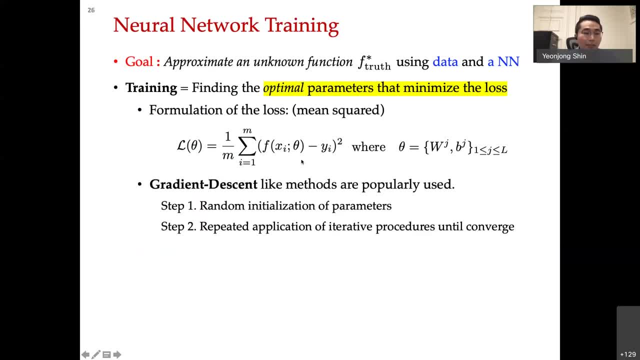 And typically this loss is minimized by gradient descent like method. And typically gradient descent like method involves with the 2 steps: Step 1. Is the random initial, Is the random initialization of the parameter. and step 2 is repetitive application of some iterative schemes until converge. 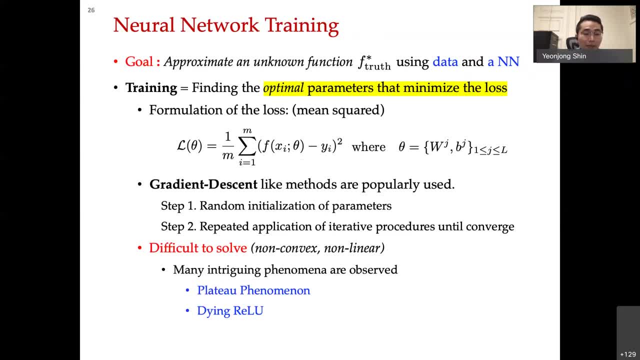 However, this is difficult to solve because it is not not convex and also non linear At the same time. this is the part where many intriguing phenomena are observed, And those are flat phenomena and the dying Ray Lou. Let me 1st illustrate. 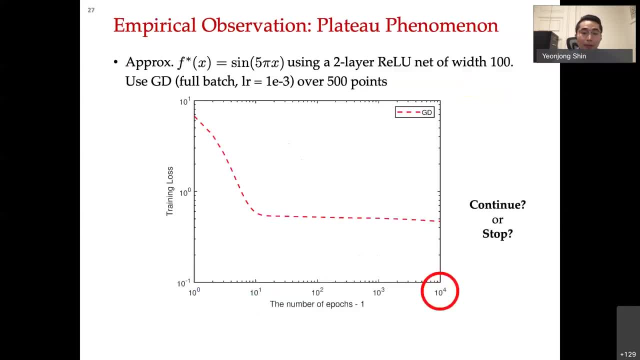 Uh, what is the flat. So here we consider uh simple Learning task, just to trying to approximate a sign function using 2 layer rail network of with 100.. And we train it with using just a standard gradient descent using full batch, and learning rate is the 10 to the minus 3.. 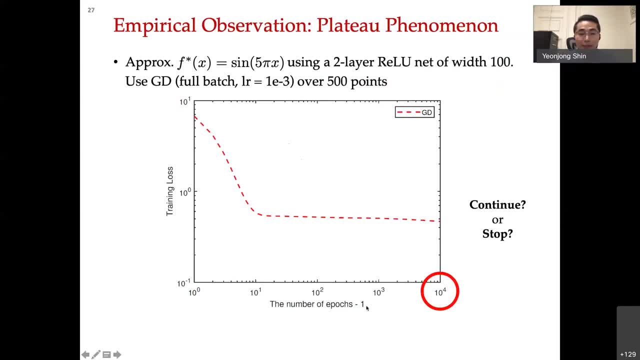 And this figure shows the training loss versus the number of iteration And we see that the loss decrease fast to get fast in the early phase And then quickly saturates and some may even think that, uh, training is done and may terminate the training at this point. 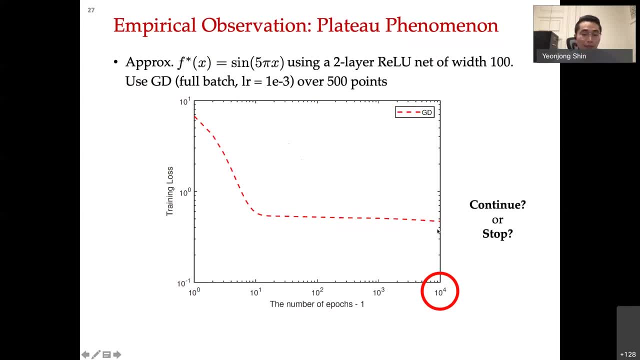 However, if we continue gradient descent, What we see is here: the most suddenly decrease, faster game People saturating at around 10M iteration, And if we go further, And if we go further, And if we go further, we see that similar behavior repeated. 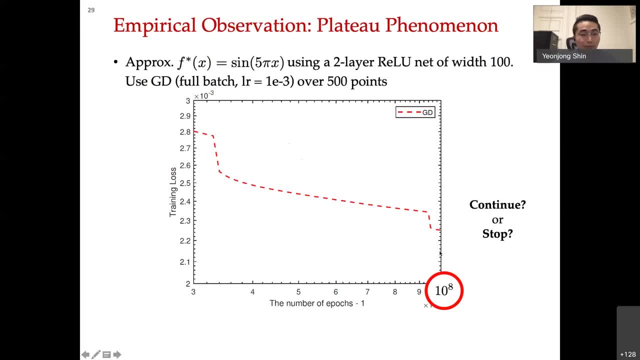 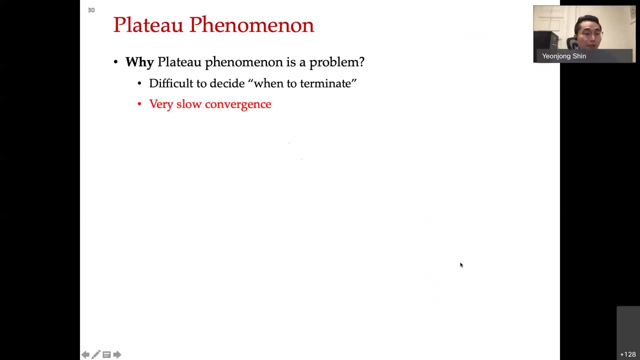 This is so called flat of phenomena. Then why is a problem? Well, as you can see, it made us too difficult to decide when to terminate the procedure, And for the more it makes the training very slow. So therefore, the goal for us. 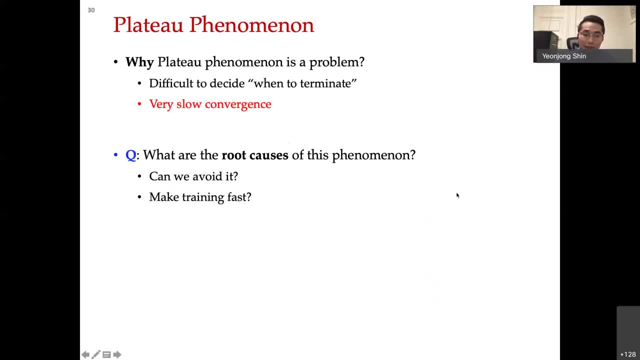 Is to understand what are the root causes Of this phenomenon. and once we identify the root causes, Then can we avoid it and make a fast conversions. I mean fast, some training method, and that was our motivation. But to address this question we need to understand some basic. 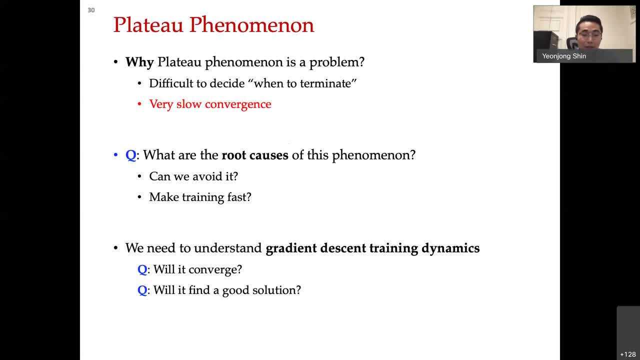 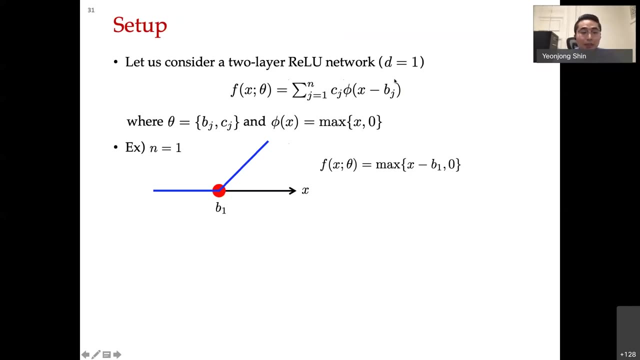 Understanding of gradient descent training dynamics. Will it converge? if it is, then will it find a good solution or not? So I will going to Go over A few more questions in SQL. Here is the cell we considered the simplest to settle we can think of, but not too trivial is the Univariate ReLU network. 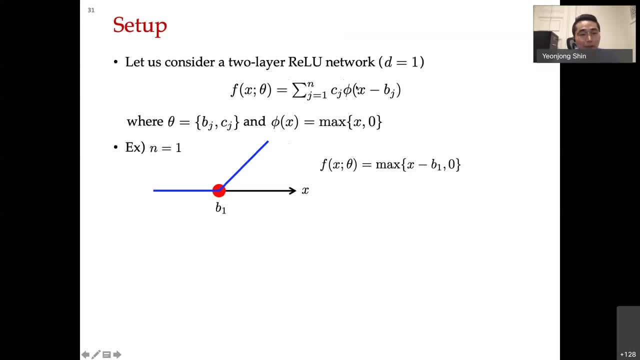 Here, which is written in the following manner- and you may notice that we don't have the W here, because the Fee is the ReLU, so that it is the homogeneous, Positive homogeneous, so that, without loss of generality, you can do this. 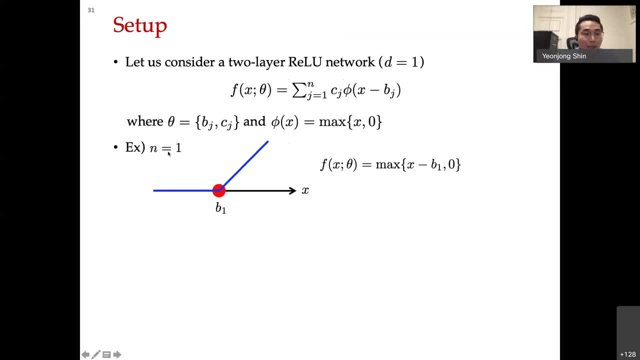 And The The other Simple. The example is that when small n equal to 1.. And the C equal to C1, equal to 1, then this is just the max function. little bit not located that B1.. And this is our 1 realization of this in your network. 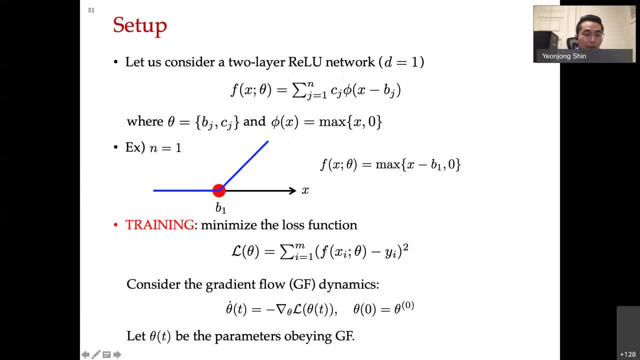 For the training, we considered the square loss function And consider the gradient flow dynamics. So from now on we are going to assume that this theta Is The Function governed by this dynamics, and this is our primary interest of the parameter. 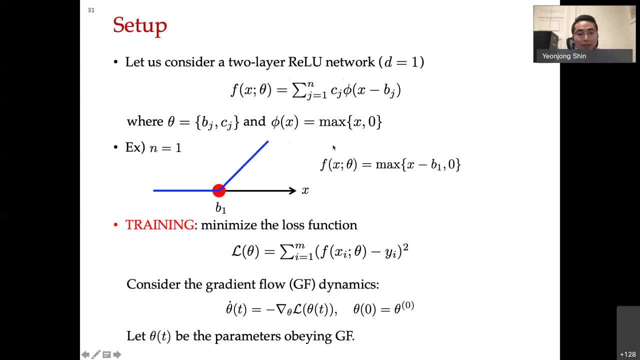 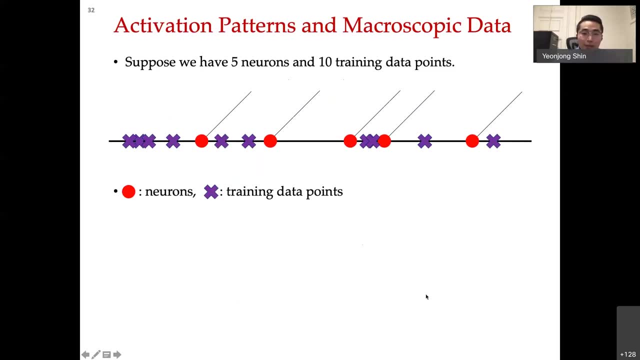 and want to know that, how this function behave as the training goes on For this analysis. there are two key concepts for understanding of this analysis. One is activation patterns, the other is macroscope data. I will illustrate what are those in the following illustration. Suppose we have five neurons which are shown as the red dots. 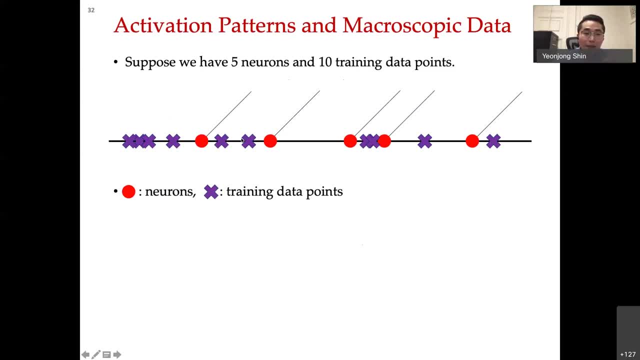 and we have ten training data points, which are the purple cross marks, Then with respect to each neuron we can define a partition of the training data. So those four points left belongs to this U set and the middle two purple dots belongs to U set. 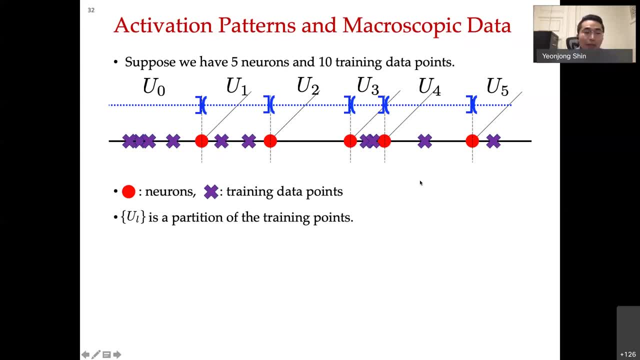 and U set belongs to this. So those left four points belong to the U set and the middle two purple dots belong to U set and U set belongs to this. set is the empty, etc. Then what we mean by activation pattern is the size of each U set. 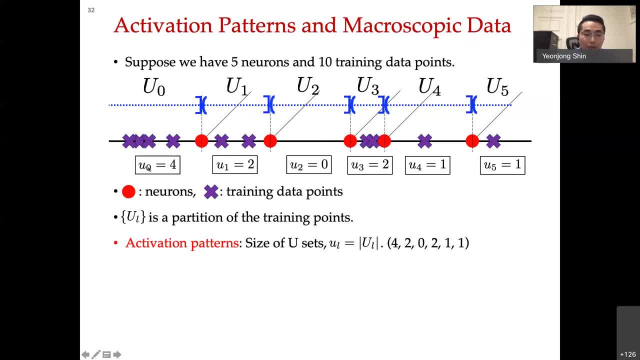 So in this example, small, u0 is the cardinality of the capital, U0 set so, which is the full, and u1 is 2, etc. And collection of all these numbers is what we call activation patterns, And macroscopic data is its corresponding averaged data. So by average of this full point, 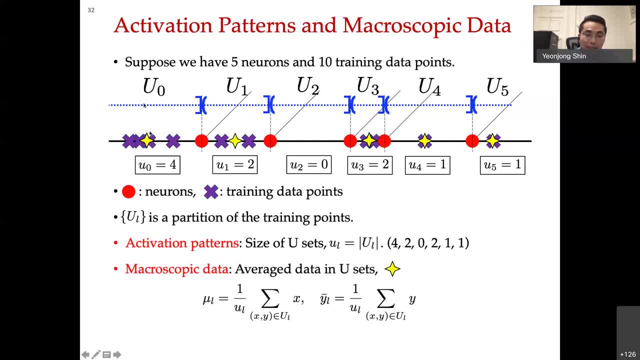 is the macroscopic data corresponding to the U0 set, and same thing for the U1 goes on. So these two are the most important concepts in understanding flat-to-phenomena and the training method that we're going to explain in later. 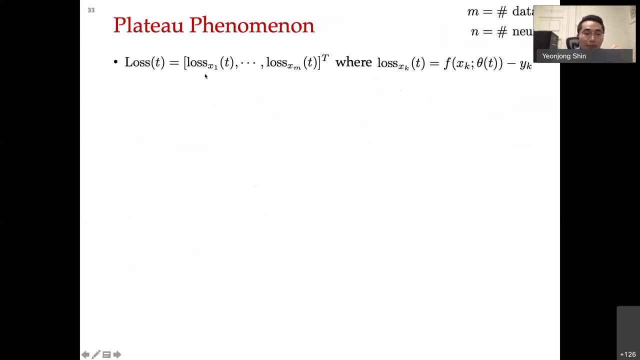 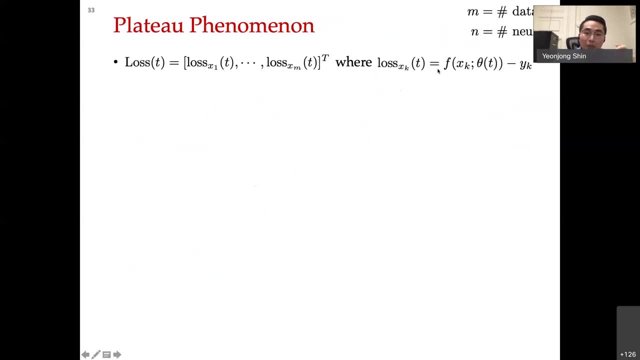 For each of the component is the discrepancy between our neural network and the output data evaluated at the case data point. So naturally, the norm of this loss vector becomes our original target loss function. The one main result is the following: For time interval on which the activation 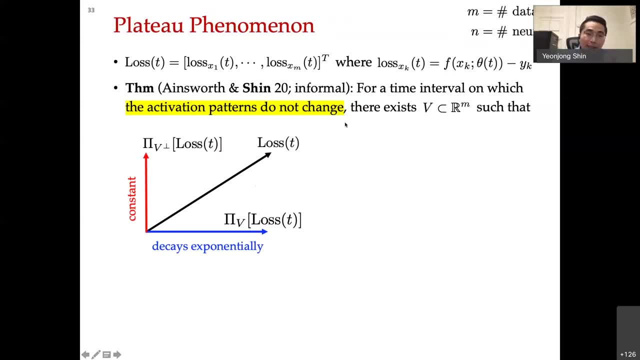 patterns do not change, there exists a linear subspace such that the loss does not decay at all in its complement space, but it decays exponentially fast on this corresponding void space. So meaning that for the time being where activation patterns do not change, 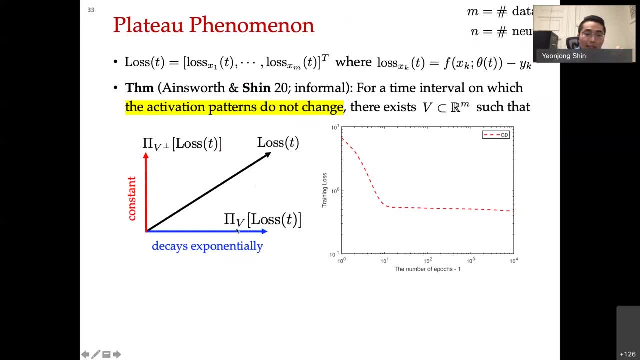 we get a fast convergence on this subspace and the rest of them are just the remainder of this part. So this plateau is converges to the orthogonal complement of the loss vector. So in other words, a plateau corresponds to a period of time during which the activation 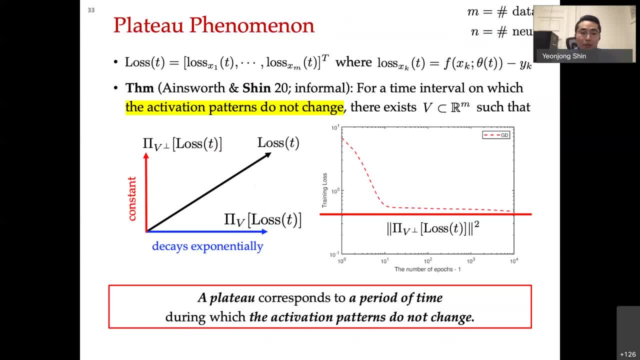 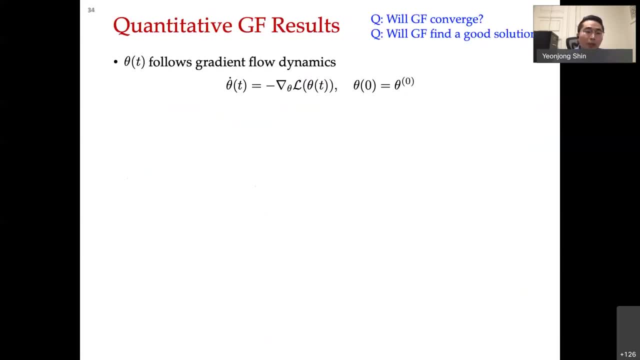 patterns do not change. So that is the root cause of why plateau phenomena occurs. And next we provide some quantitative result of the gradient flow. Mainly, will gradient flow converge or and the will gradient flow find a good solution or not? So again, theta t follows these following gradient flow dynamics: 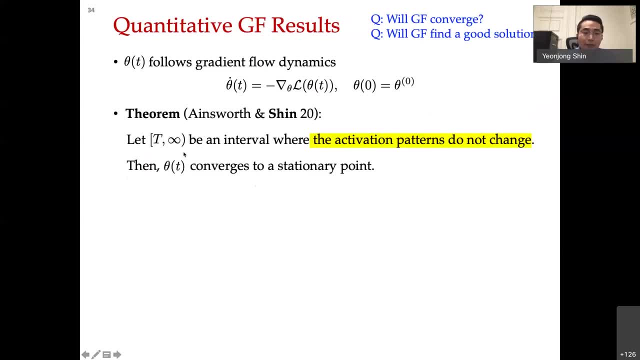 And the one partial theorem. the partial convergence theorem we prove is the following: Suppose that there exists a time interval, t, from infinity where activation patterns do not change, Then theta t converges to a stationary point. Then this provide the partial convergence. 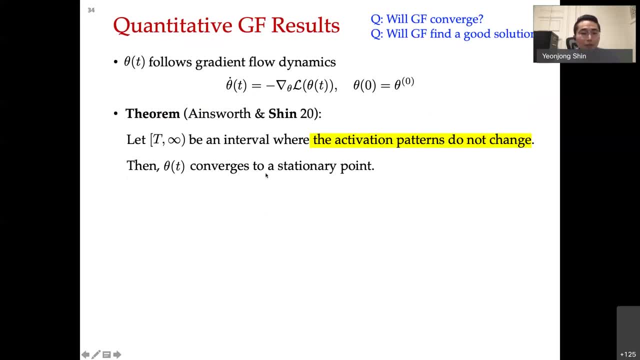 The next question is then: what is the stationary point and how it looks like? So we quantified the if and only if condition for a point being stationary, but I want to emphasize just one thing on this lemma: This condition shows that fully trained network interpolates macroscopic data. 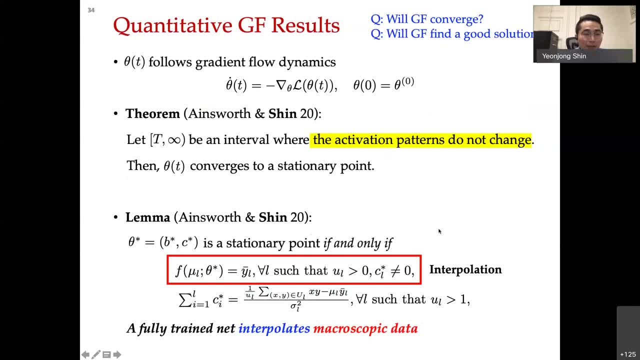 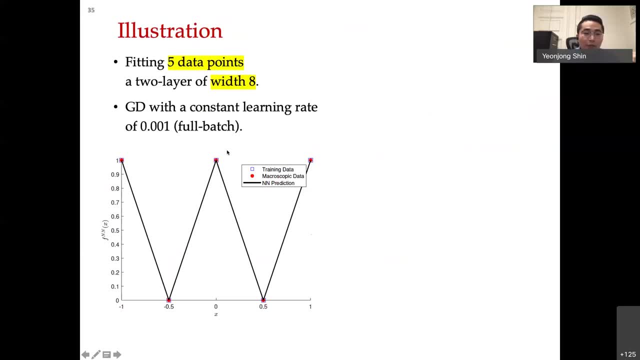 I will going to explain this theorem and lemma in the next slide here. First, we are trying to fit the five data points shown in here: 1,, 2,, 3,, 4, 5 is a double shape and we train with the ReLU network of width 8, just GD and constant running rate, et cetera. 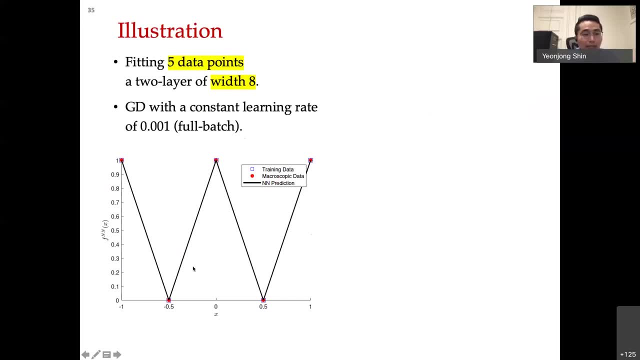 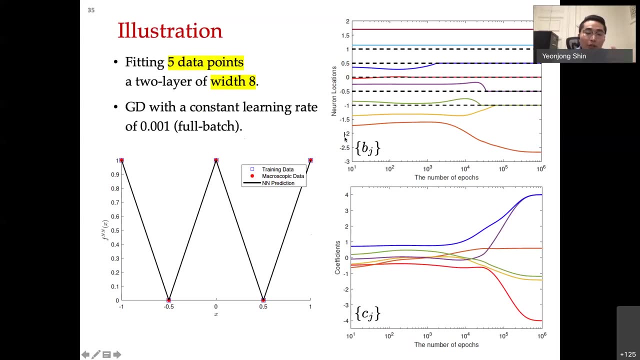 And you can see that fully trained network interpolate all the macroscopic data which is shown as the red dots here And here. furthermore, here we show the training trajectories of the biases and the coefficient with respect to the number of iterations, And here black dashed line corresponds to five data points. 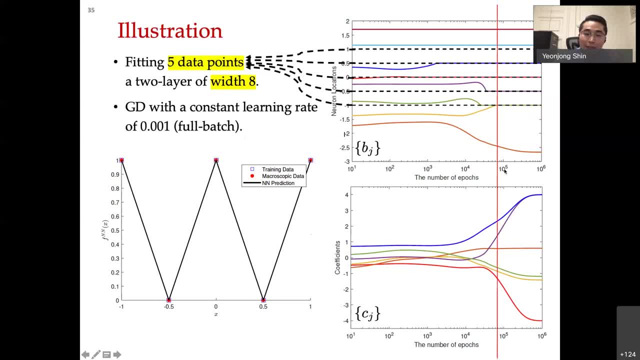 And what we can see here is: at around the 10 to the 5 iteration, you can see that all the biases are somehow stabilized, which meaning that we have fixed activation pattern. afterwards Meaning that after 10 to the 5 iteration, for the rest, we have a fixed activation pattern. 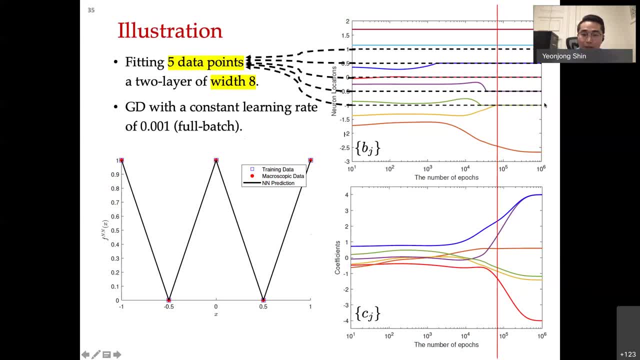 so that we should expect to have conversions Based on that, Based on our theorem. And this is what's happening, as you can see in the coefficient: Once the biases are stabilized, now coefficients become converged and we have reached the convergence. And also one thing is related to the later dying ReLU. 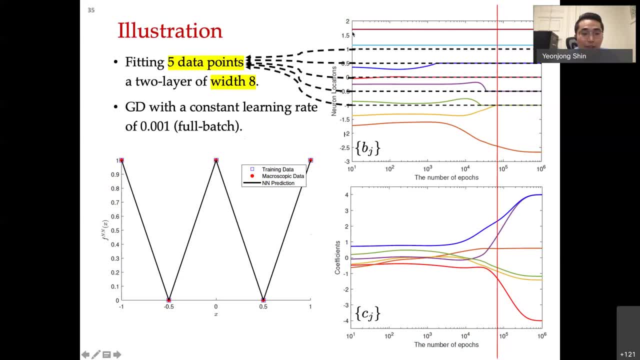 You can see that these two upper two does not change at all during the training, And this is because of the dying ReLU, which I will going to explain in the last topic. All right, Then now. So we have to look at the next step. 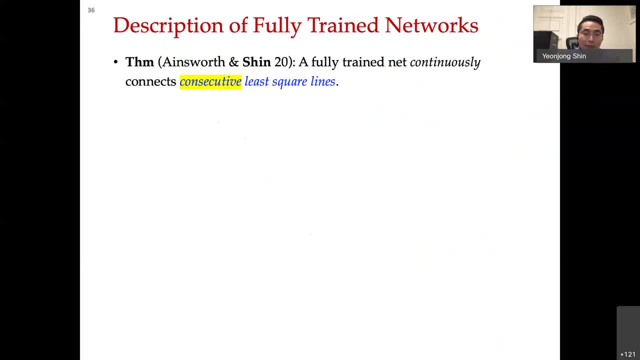 So we have to look at the next step And that: will gradient flow converge or not, and how it looks like? And the final result is the this: Will gradient flow provide a good solution or not? And here is what we proved: A fully trained network continuously connect consecutive least squares line. 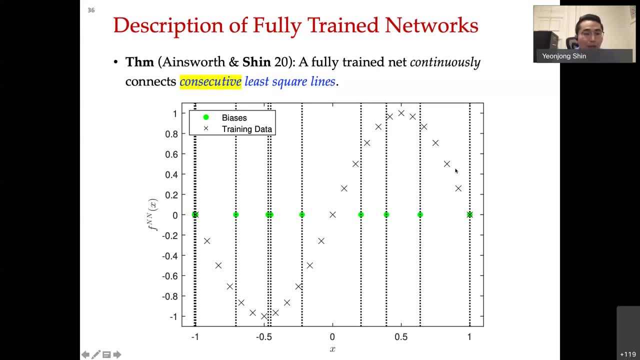 So let me explain what it means in this flow. So marks, our training data. Then we focus on just the UJ set, which is the interval that corresponding to interlaced of the consecutive neurons. Then, by focusing only this, relum, 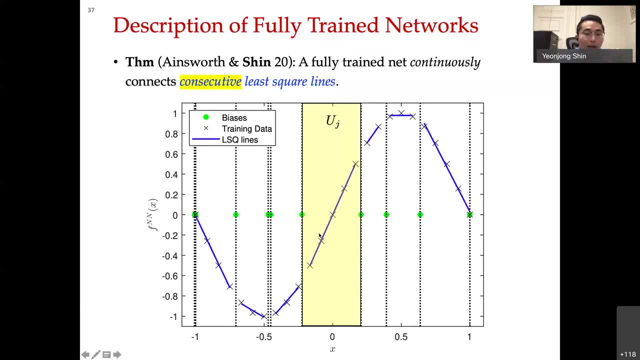 we can just fit a least square line by using those five data point. And same thing can be done for other relum And its macroscopic data is the red dot. so the least square line actually passes through this macroscopic data. And what fully trained neural network do is. 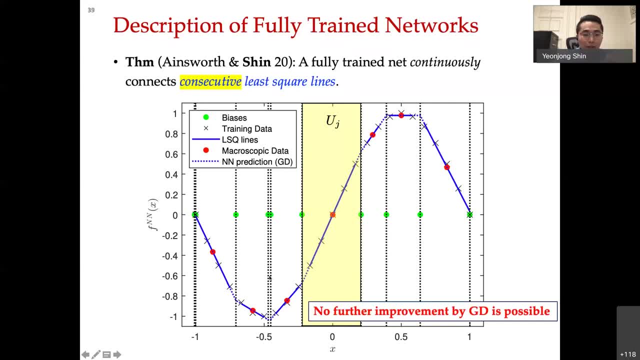 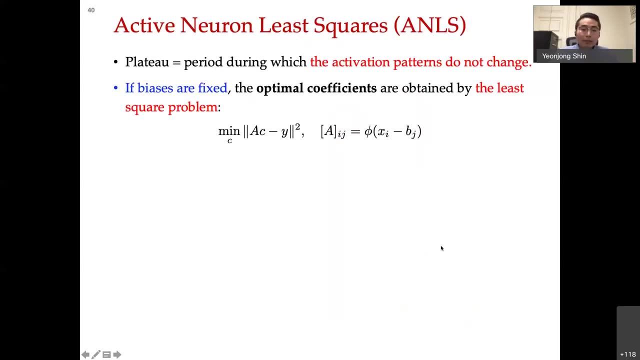 continuously connect these least square line, What the flow and gradient descent training do, and at this moment no further is possible by gradient descent. All right, Then, all these theoretical result we gained provide some insightful result. So one is: the plateau is the period during which the activation patterns do not change. 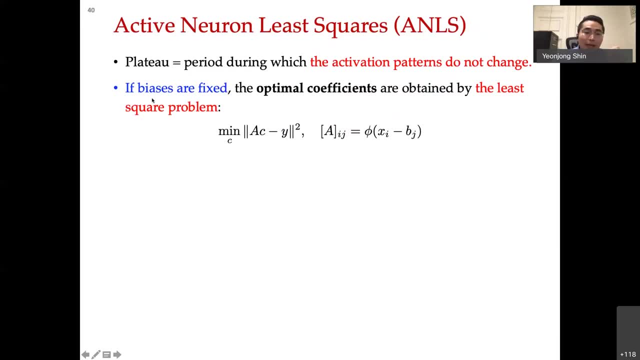 And the second observation is that once biases are fixed, the optimal coefficients can be obtained by solving the least squares problem And this combine these two and we can get a new training method which is we call active neuron least squares. The idea is that we 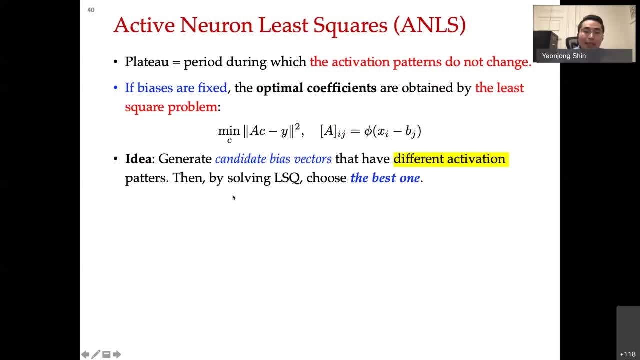 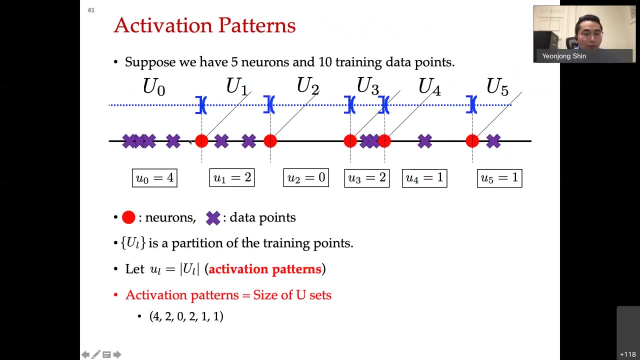 want to generate candidate bias vectors that have different activation patterns. And then we solve the least square and choose the one with the smallest loss value. And here let me quickly recall you what was the activation pattern? So, given the five neurons here, and each neuron actually- 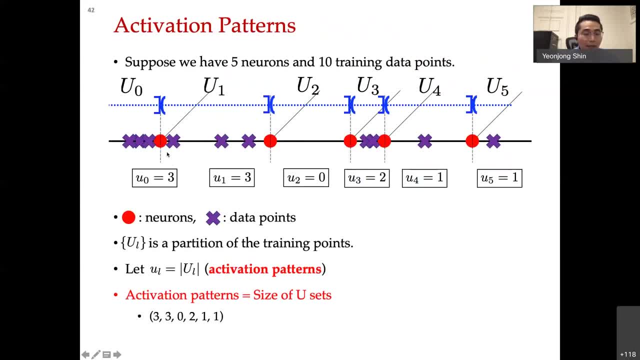 Okay, Okay, Okay, Okay, So we can actually partition the data and the collection of these. the size of each U-set constitute what we mean by activation pattern. Then actually we can manually change the activation pattern. For example, if we move the first neuron to the left, then this creates the new activation. 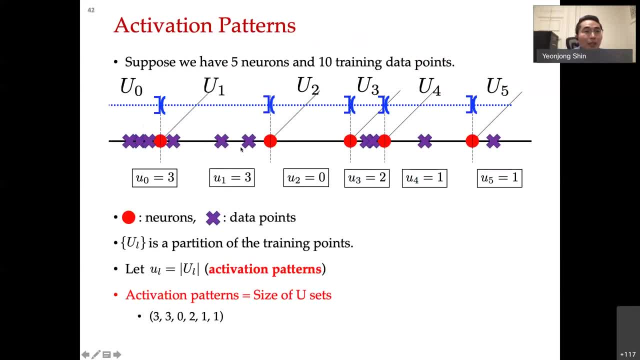 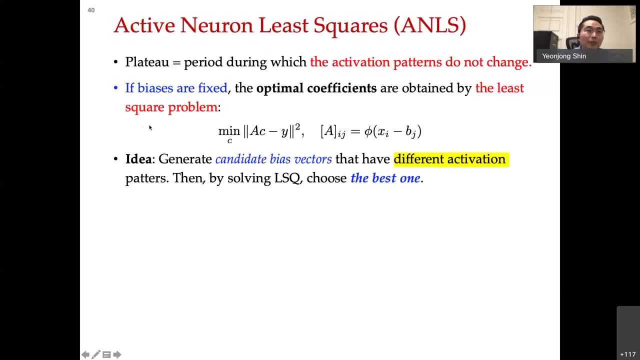 pattern. So you can see that here is a number of. the data point of U0 set was full, but by moving the first neuron the data point was full. So if we move the first neuron to the left, oops, we get the U0 set becomes three U1 set. 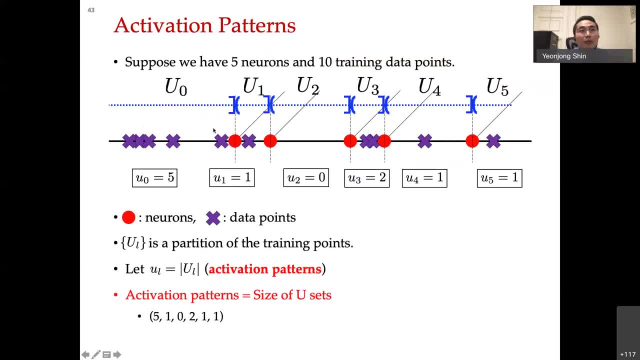 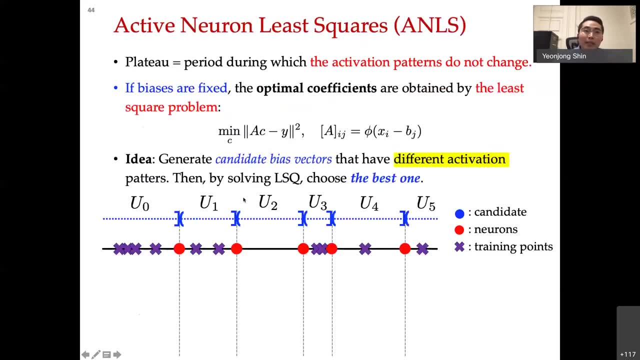 becomes three And do the same thing. if we move the first neuron to the right, then we got U0 set five and U1 set one. So in this manner we can create multiple candidate vectors. that generates a different activation pattern. So this is the one example. another example: 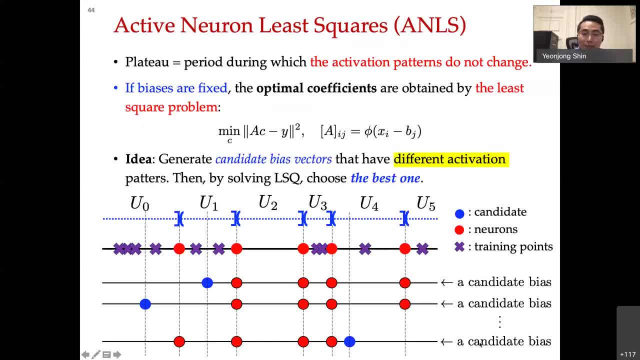 et cetera. Then, among all these different candidate bias, we get a different activation pattern. So we can actually use the same method to create multiple candidate bias. So we can actually use the same method to create multiple candidate bias. So we can actually use the same method to create multiple candidate bias. 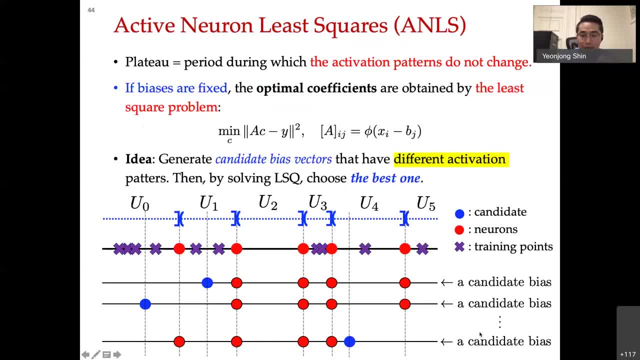 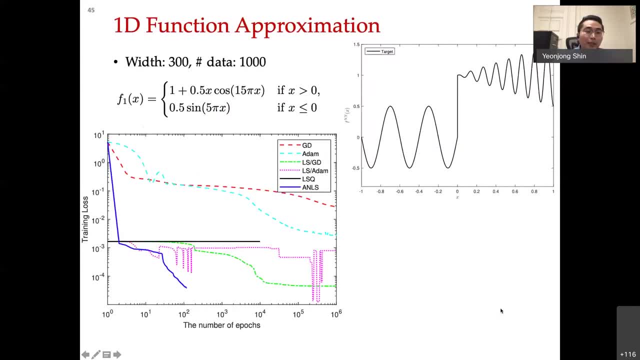 Then we choose the one with the smallest loss value And we have a very efficient procedure of choosing the best one. but let me skip that one and show the performance. So this is the 1D function, approximation task. So this is a target function. It's a discontinuous Left. one is the low frequency The right one. 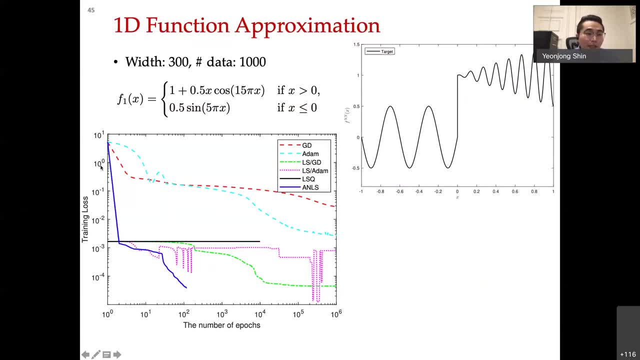 is somehow high frequency here. And here is the training loss versus the number of iteration And we compared with the gradient descent ADEM and so-called LSDD, LSADEM. So applying least square and gradient descent ADEM iteratively, And the black solid line is just the standard least square, right after the. 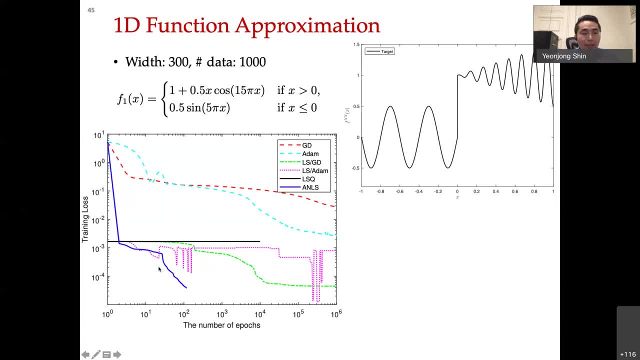 initialization And the blue one is the training rejected by active Newton least square. You can see that with a merely 100 iteration it already achieved the best training loss And also in terms of the training loss. it achieved the best training loss And also in terms of the training. 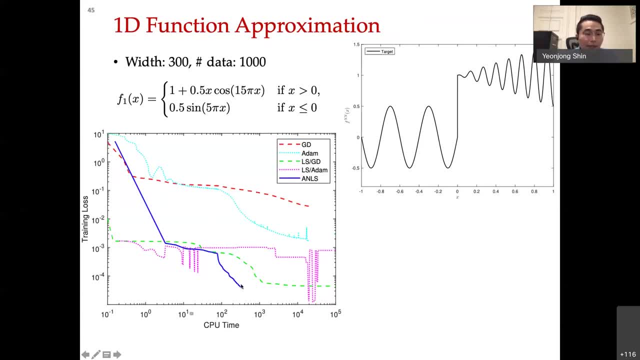 loss. it achieved the best training loss And also in terms of the CPU time also is the shortest time and get the smallest loss. And what about the generalization error? So here I show the prediction error here And you can see that an active Newton least. 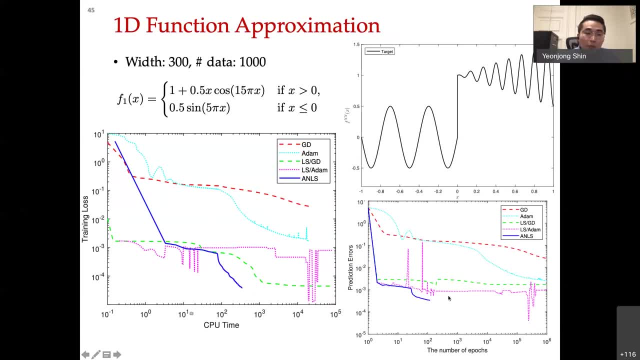 square achieved the best result. among others, One particular thing is the following: If you see the green dashed line and our blue line, you see the training error is roughly the same. However, when you see the prediction error, active Newton, least square actually. 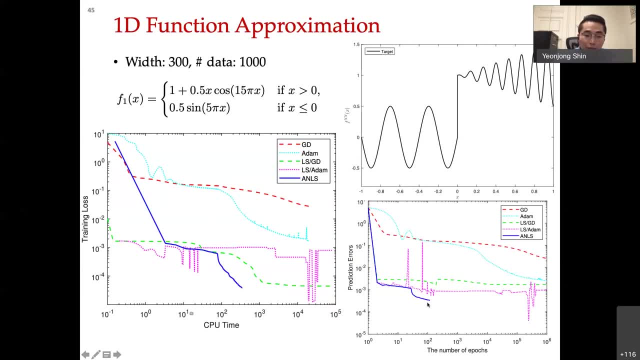 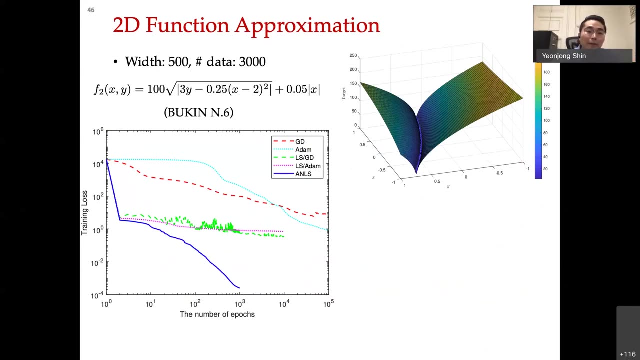 produced a more great result on the generalization performance. So active Newton least square also generalizes well, And we also extended this method to the multiple dimensional task. So this is the one example for the 2D function approximation. The target function is so-called the booking. 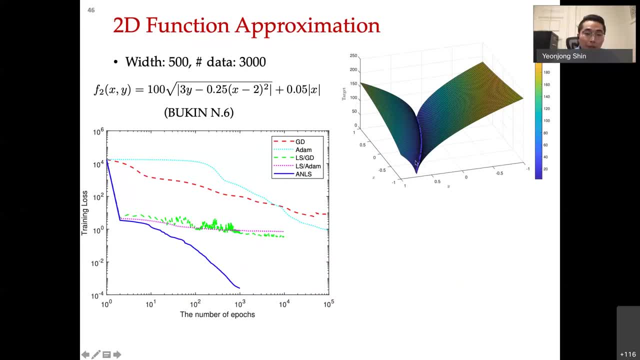 function, which is quite a difficult function to be approximated, because if you see the values of the function, it goes up to 0 to 200.. And also you see that there is a shock belly in here where the somehow non-differentiable part has appeared. 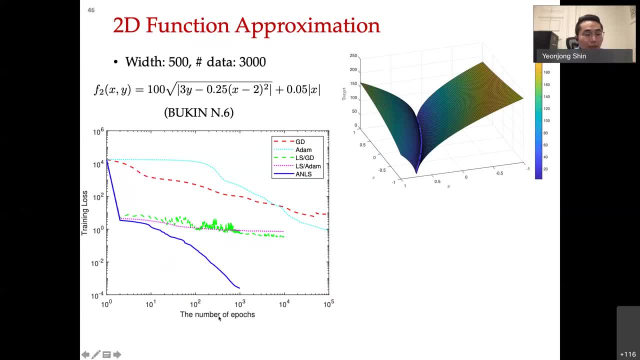 And here you show the training loss versus the number of the iterations. You can see that active Newton least square, performs roughly four orders of the magnitude better than any of the other methods. And this is also CPU time. and also not to mention about the generalization error. 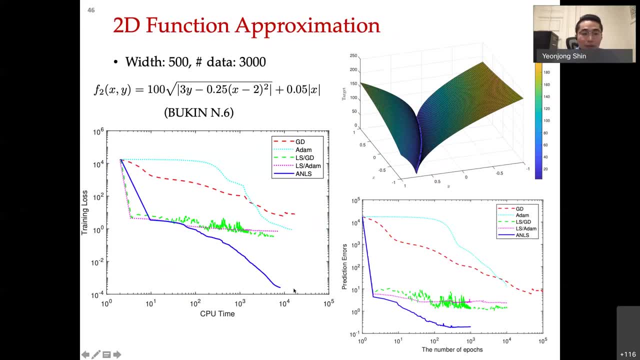 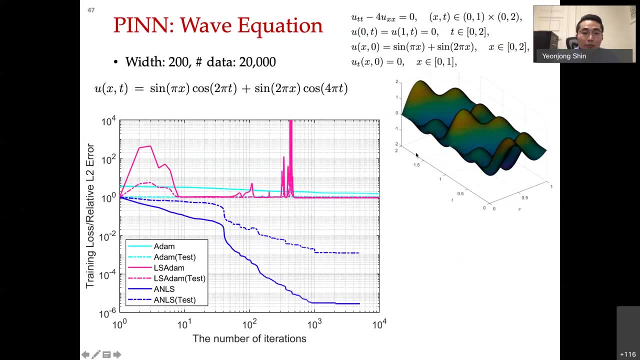 Achieve the smallest generalization error and the smallest training loss, And this can be readily applied to solve the PIN. So one of the bottleneck of the PIN- some might people call this the- it's hard to optimize or there are multiple some issues. But 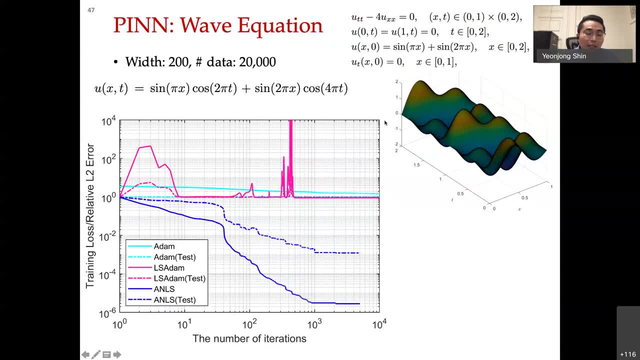 without changing any activation function or without changing any neural network architecture. we just use the two-layer neural network and, trained with active Newton least square, we can solve this wave equation and we can see that it's working nicely. And here I show the training result and the relative L2. 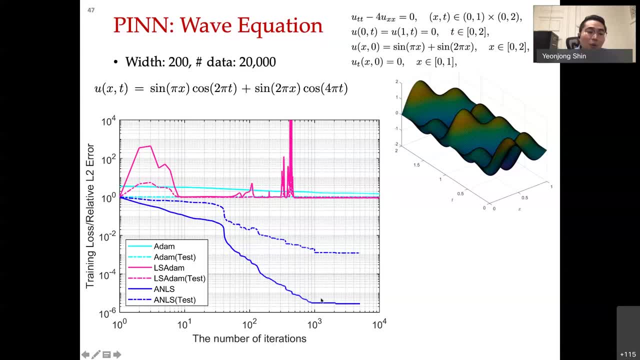 error. Relative L2 error is shown as the dashed line And you can see that active Newton least square is the only method that works. None of them are working really well but achieved a 10 to the minus 6. training loss and relative error is roughly 10 to the minus 3 level. And here is the 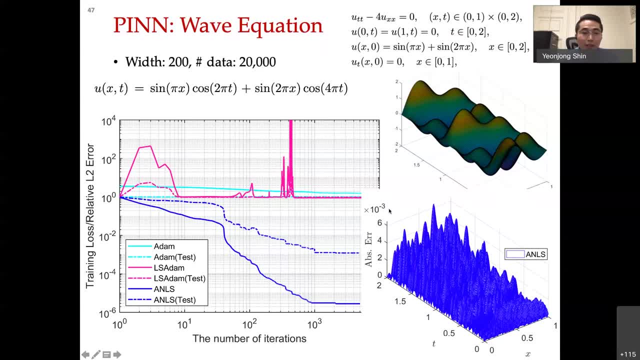 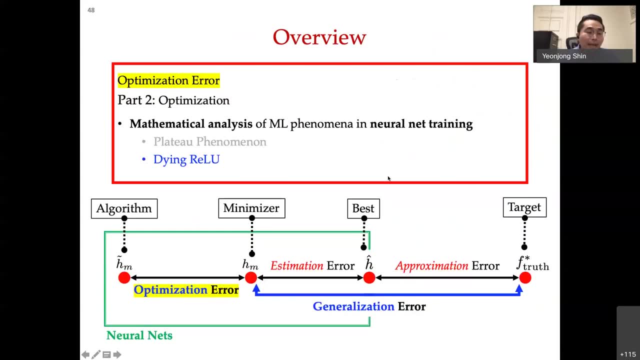 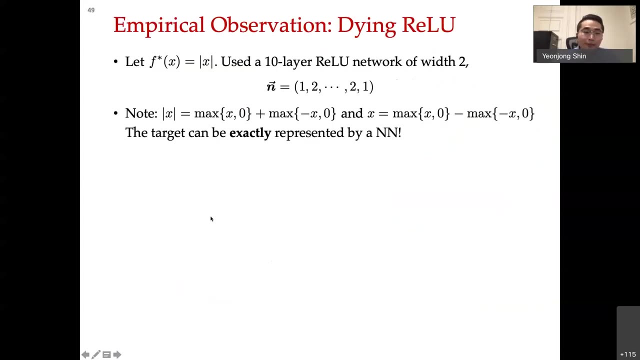 absolute value error plot on the domain for the wave equation. So that was the plateau phenomena And the last one is the dying ReLU. So let me illustrate what is the dying ReLU. So suppose we want to approximate the absolute value of X, which is simple function. But someone said the DIM neural network is very powerful. 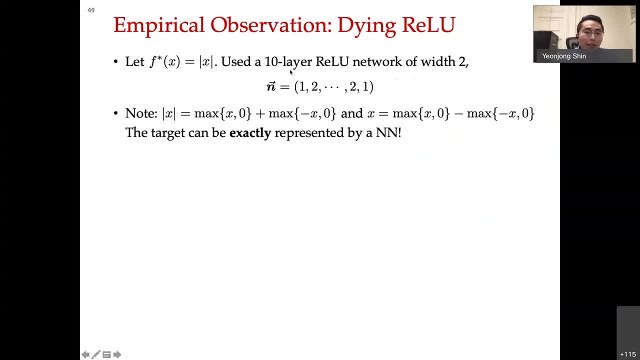 So suppose you want to use the 10-layer ReLU network of width 2.. Theoretically this neural network is powerful enough to exactly represent this absolute value of X because of the following relation: So absolute value of X is just the addition of the two. 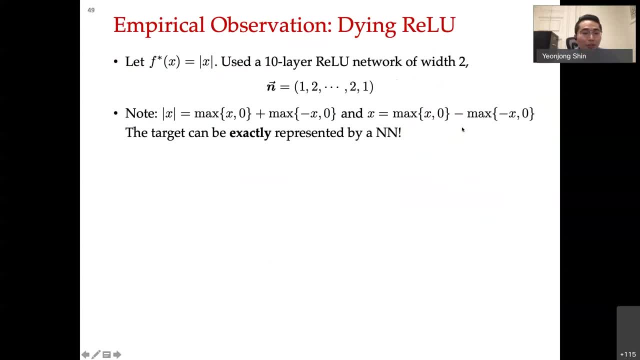 neurons. Identity map is also addition of the two neurons so that you can just decompose absolute value of X and just identity map recursively. So target function can be exactly represented by a neural network. But when you actually train it Then what you get is 9 out of the 10 times. you see that this 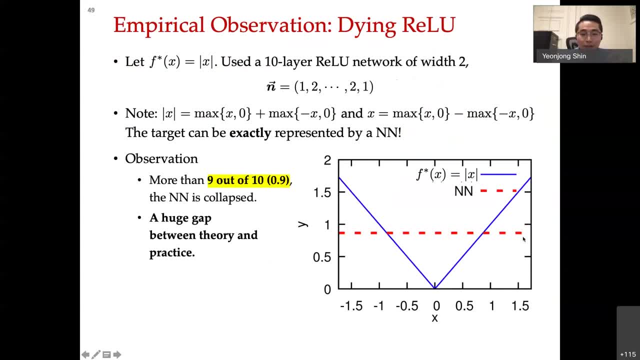 Flat dashed line. so this is the train to reject And this, the blue line, blue solid line, is our target function. So you can see that clearly there is a huge gap between theory And practice and, in terms of this, the diagram that I show you earlier. 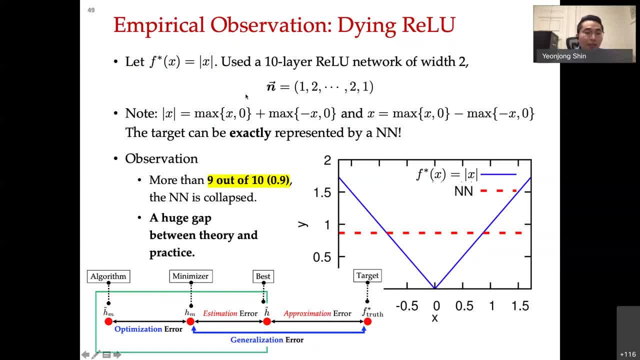 There's no approximation error because it can be exactly represented by this: The 10 layer with two relative network, the target function. So there is no approximation error And also there's no or negligible estimation error because We train it over 3,000 training data or 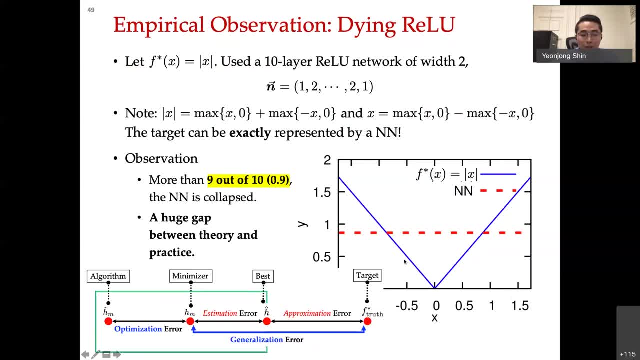 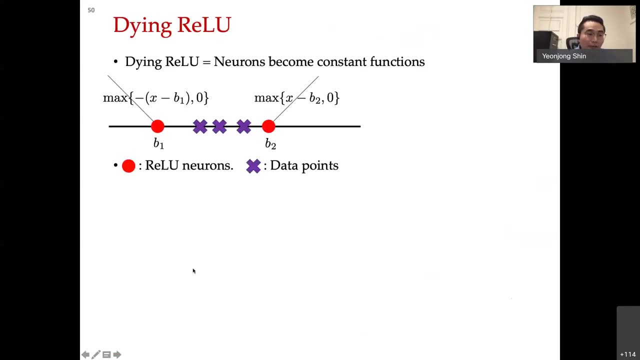 more for only just approximating this simple 1D function. So generalization error is negligible or none. So this is mainly because of the optimization Negation error and what's happening here. So dying really is our reason why it is happening. 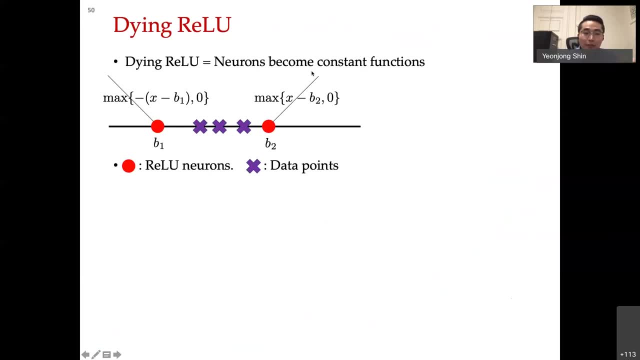 So that really, in simple words, neuron becomes a constant function. So this is the one some illustrating example. Suppose you have two railing neurons going, this word and that word, And if your data point lies between this, then when you evaluate this data, 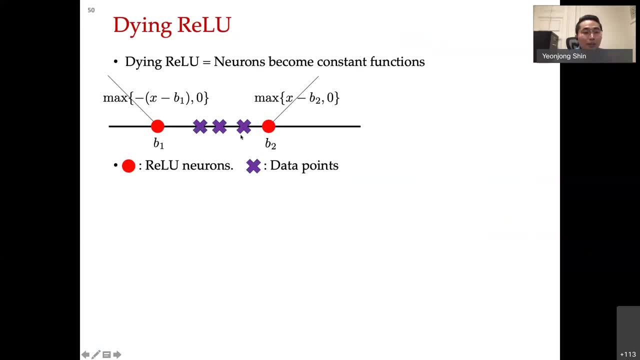 These neurons on this data point, it becomes all always a zero. So why then? why? this is a problem because we use the gradient to base the training And gradient of the constant function is a zero, so gradient descent does not work. So this is the simple explanation of 1D parameter set, set up. 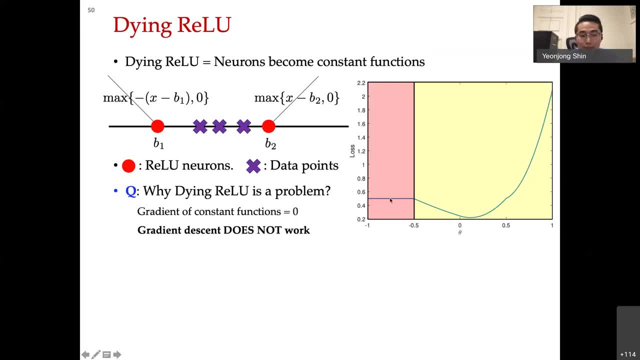 So if we start with this red realm And you'd apply the gradient descent, It doesn't update at all and just stay there and just nothing happened. So the question is then, in the more general setup, what, how likely we start our initialization in this red realm? 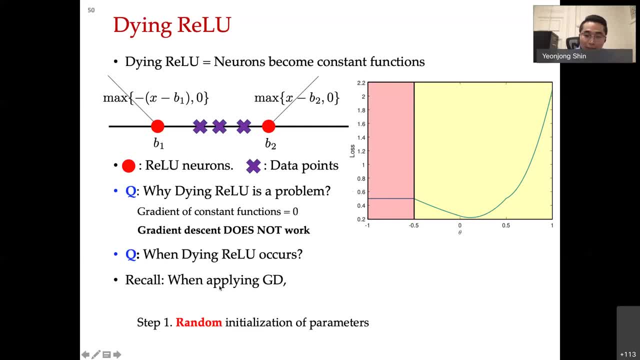 And recall that when applying gradient descent, like algorithm, we randomly initialize the parameters. But 1 thing we often forgotten is the step 0.. We need to, We need to choose a network architecture. Which network architecture would be more preferable? And what we quantify is definitely depending on the depth and the width. 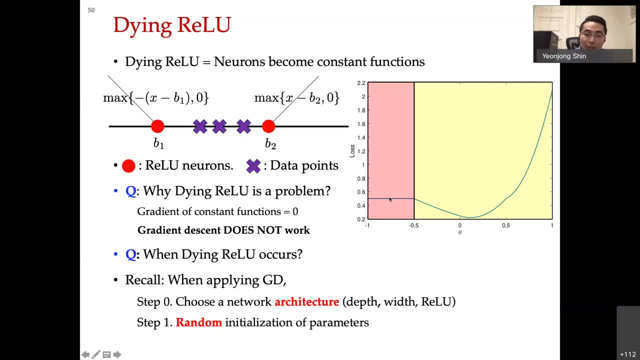 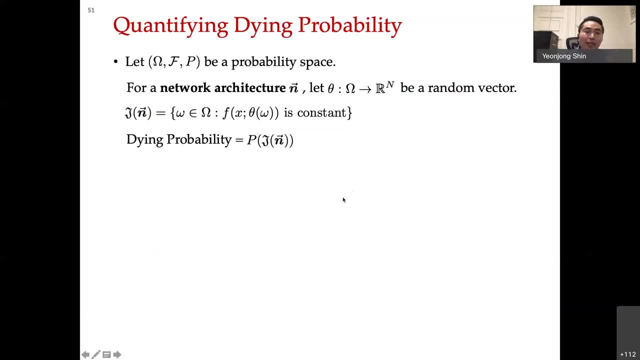 The probability that you start with your optimization in the red realm actually changes. So to this end, we want to quantify dying probability. So, more rigorously, we define some probability space And, given the neural network architecture, Then we define the event where network become a constant. 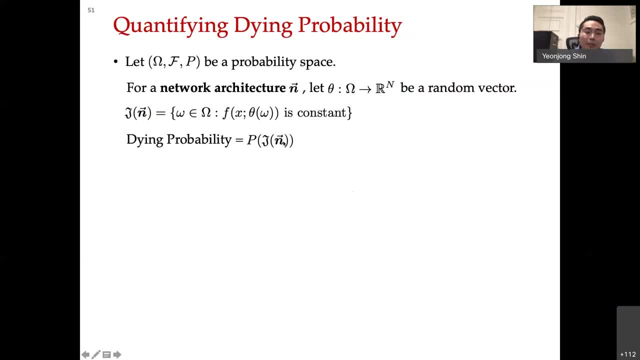 So we want to identify how likely this time probability would be depending on your network architecture. So 1 asymptotic result we show is the following: given on your network, in your network, And suppose your network parameters are ID from symmetric distribution. 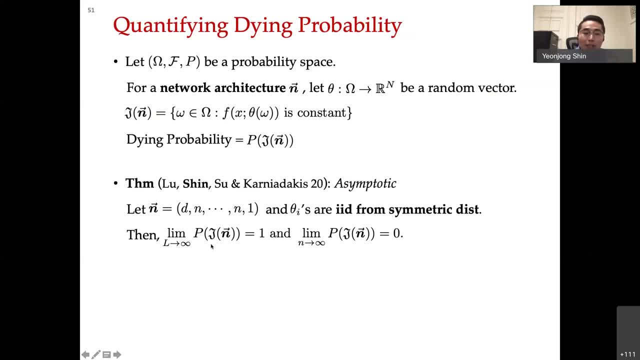 Then Dying probability goes to 1.. If you fix the width and let the depth goes to infinity, And for the more, if you fix the depth and the width goes to infinity, then this dying probability is a 0.. And this is somehow explains why in practice, the wide network is so successfully used and not deep and narrow network. 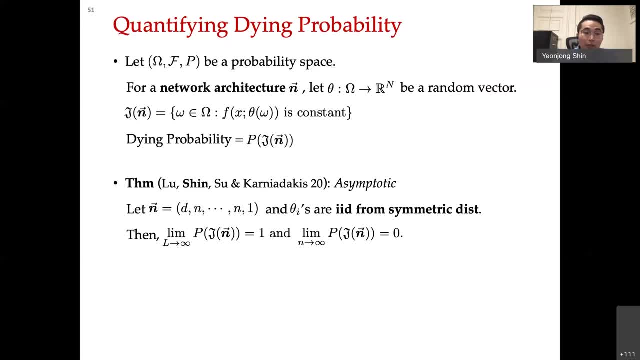 Although deep and narrow network enjoy some quite useful or theoretical guarantees. So, in simple words, Probable explanation on when dying rail occur. Simple words: deep rail network will eventually die in probability, While a wide rail network will not die in probability. 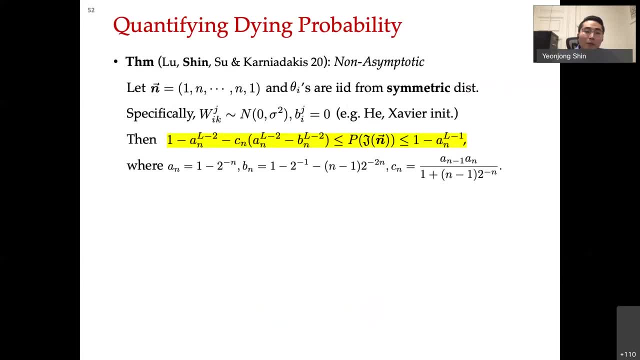 So this is asymptotic result and we can go further to provide the known asymptotic result. And here we assume some standard assumptions: The double, the weight metrics- These are from Gaussian- and is 0. Which is the common in practice. 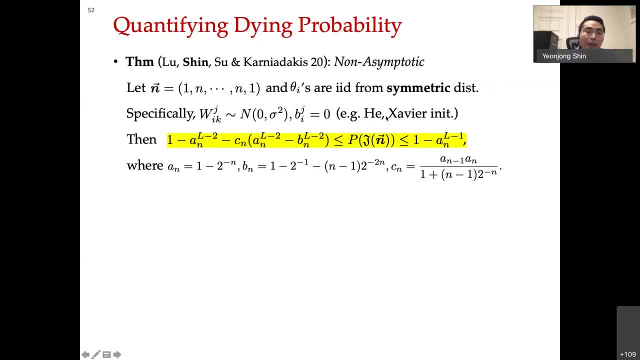 such as the He initialization or Zeger initialization, But we have somehow restrict ourselves to the one-dimensional case due to technical difficulties. But to the end, what we can get is the lower and upper bound simultaneously, And this can be illustrated by the following figure. 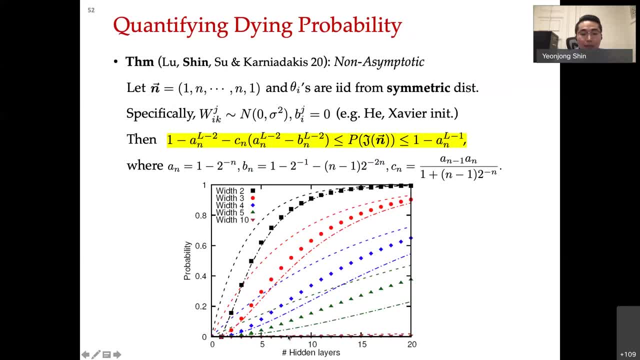 Here we show the dying probability with respect to the number of hidden layer at different width: 2 to 10.. Upper and the lower dashed lines is coming from our upper and the lower bound And the solid mark are our empirical simulation obtained from 1 million Monte Carlo simulation. 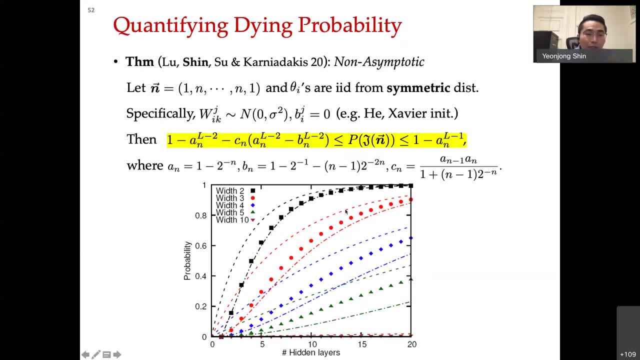 And one particular thing: you can see that these two bound are pretty accurate to capture all the reject And, in particular, when the number of hidden layer is 10 and the width is 2, we can see that dying probability is 0.09.. 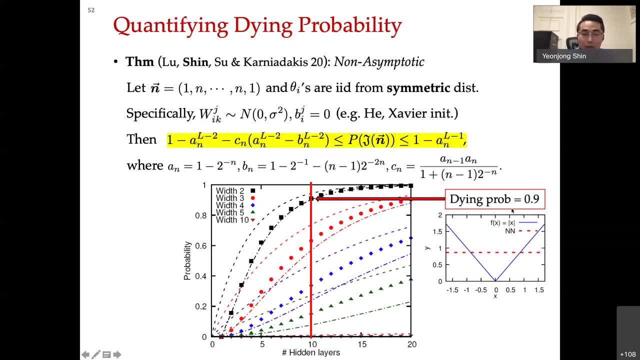 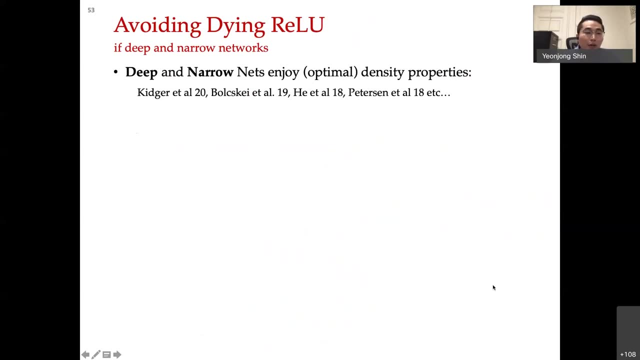 Which is same as what we empirically observed. So this is accurately predict what we have observed in practical situation in approximating absolute value of x. OK, Then now how we avoid dying Rayleigh. There are multiple choices. you can avoid the dying Rayleigh. 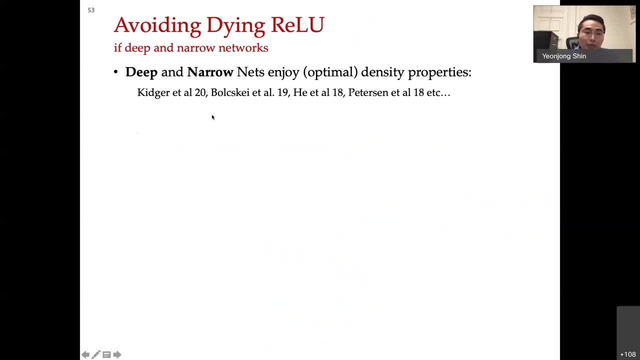 But if you want to use the deep and narrow network, then there are other option we propose. And why deep and narrow? Well, it enjoys some optimal density properties And that's why it's so important, As proposed by many methods, For example, key building block of showing. 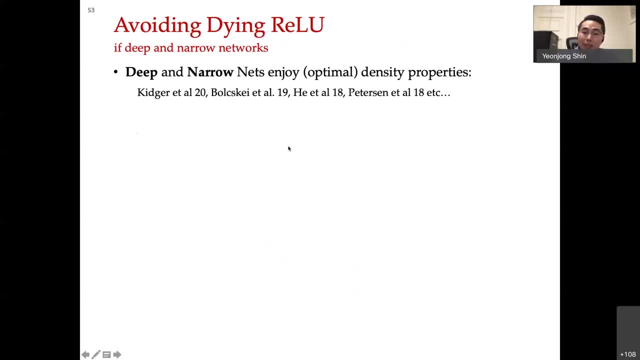 the universal approximation theorem is: construct a multiplication operator. And if you look at how those network are constructed, they are in their fundamental level. they construct the deep and narrow network And to this end, what we have proposed is the randomized asymmetric initialization. 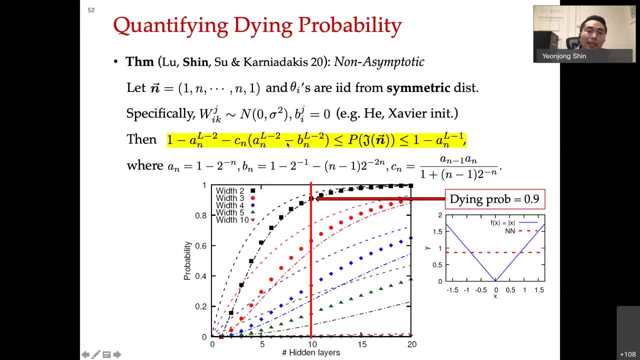 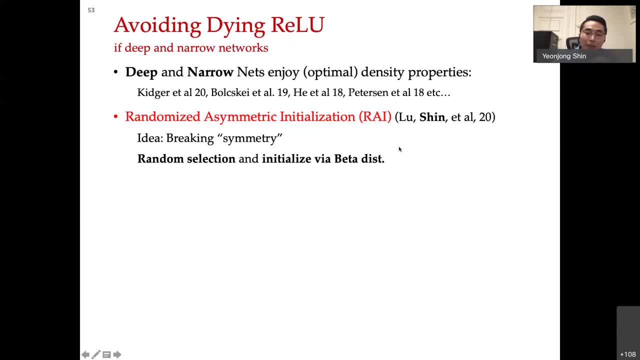 The idea is breaking the symmetry, Because all the existing methods utilizing the symmetric distribution- Actually the symmetric distribution actually in fundamental reason- why we often faced is the dying Rayleigh, especially when the number of the depth goes large. So idea is the random selection and initialize. 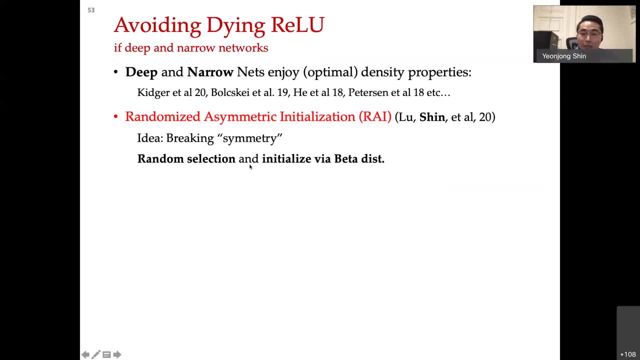 via specific beta distribution, And this can be obtained theoretically by controlling the expected square length of the output, which is the length of the network. Then, by utilizing our proposed method, we can drastically reduce the dying probability. So here is the dying probability, with respect. 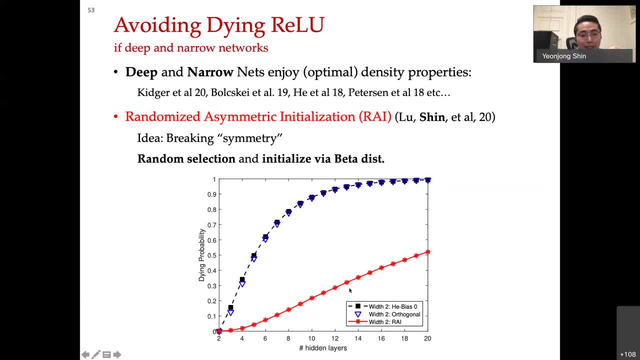 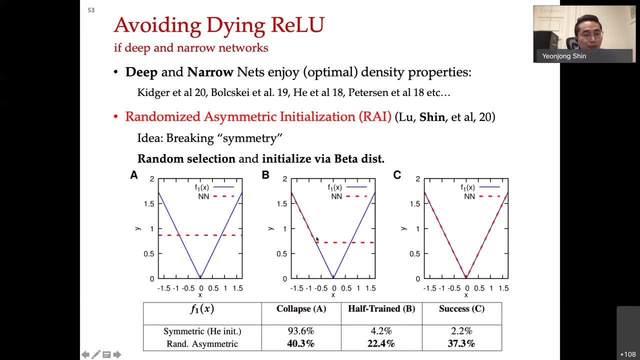 to the number of a hidden layer, And here is the width. two And red line is the one obtained by our reject And the he initialization and orthogonal initialization are doesn't very helpful in reducing the dying probability, So we're going to explain the deflection of the die and a 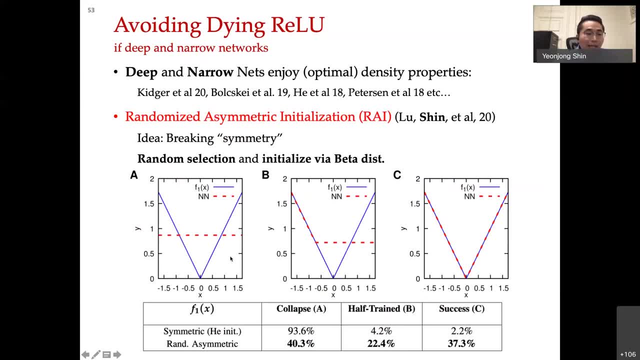 in this step, And so we have represented two sets of values for the dwelling of the die. We have the value of X, which is a parabola, and a Katie, So we have the value of X. It's a pretty simple, yourselves. 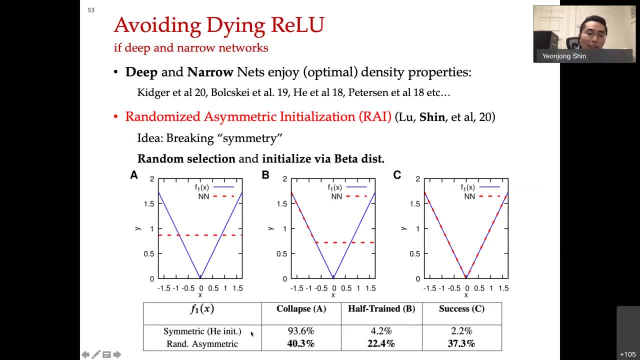 Here is what the result is. Here is the total value of X And we have the absolute value of 2.. So the actual value of X, the step appreciated by the learning test, And we have the value, And then we have the absolute value of the training. 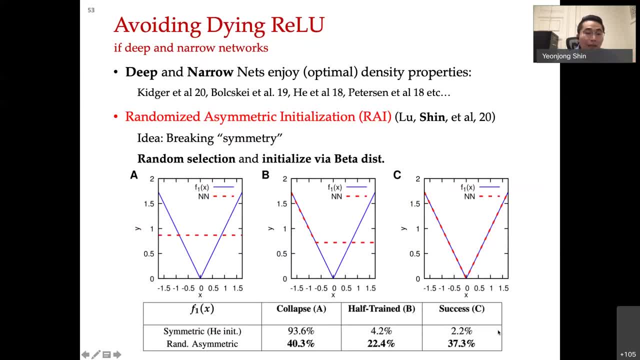 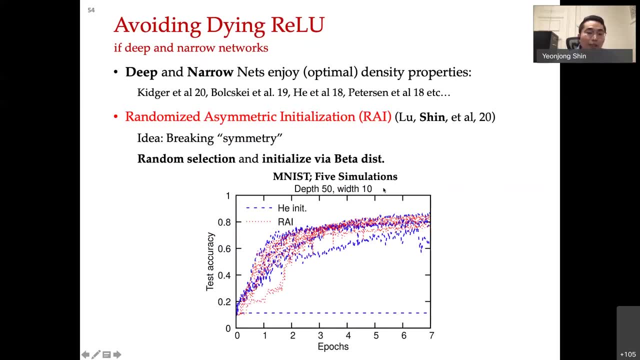 Here I show the same learning task of approximating And we also apply this initialization technique for the MNIST test and five independent simulation. We see that all the results initialized by the randomized asymmetric initialization produces the all good result. However, just using he initialization you can see that you may face in some failure of the training and some test accuracy is deteriorate in some cases. 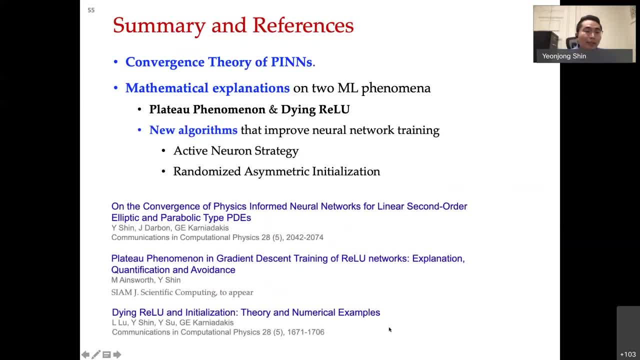 Okay, so here's the summary. So I presented the first convergence theory of the physics-informed neural network is based on the Felder regularization method And this provides a consistency result of the physics-informed neural network. So basically, mathematically it will give you the correct answer if you can get a good optimizer. 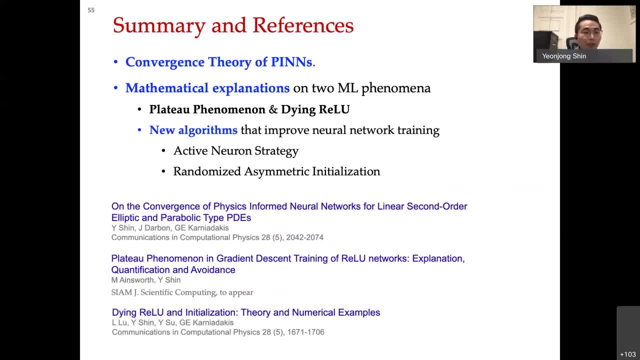 And next I discussed some optimization perspective and explained two machine learning phenomena Coming from training neural net. One is the Felder phenomena, the other is the dying-ray loop And, based on the theoretical understanding, we proposed the new algorithms that improve the training of the neural network. 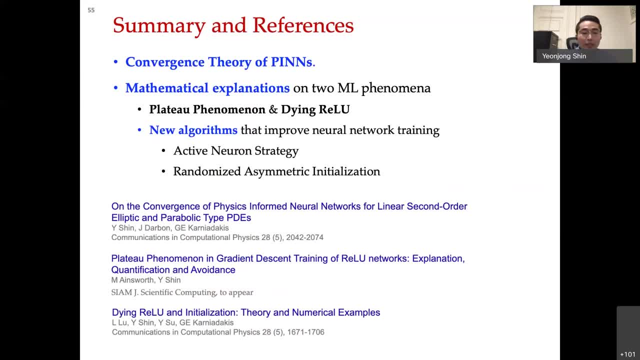 One is the active neural NIST squares. As you can see, it drastically improved the training performance And just in the, for example, the pin example is a solvable versus not solvable case And for the dying-ray loop we proposed the randomized asymmetric initialization. 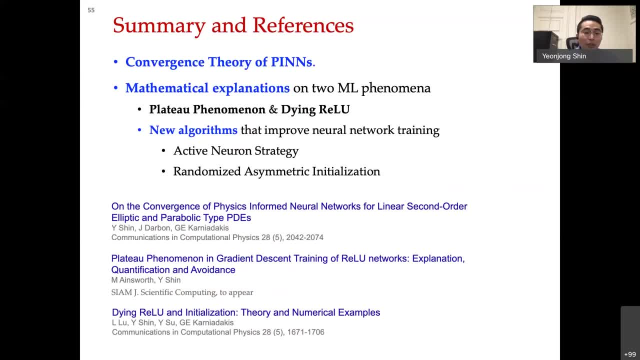 So that this allows you to explore some options of using deep and narrow network in particular cases, And here are some references And that's what I have prepared for today And I'm happy to take any questions, Thank you. Thank you so much, Yeonjung, It was a wonderful talk. 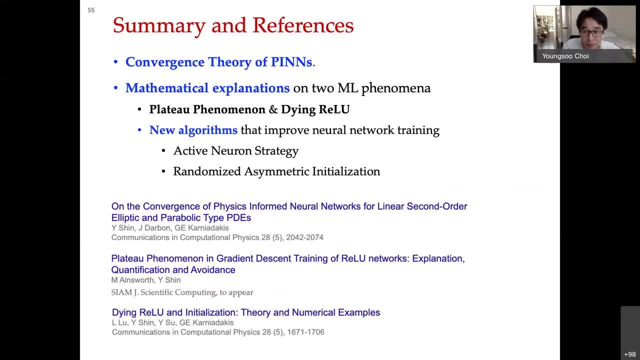 Although it was theoretically oriented, I was able to follow. clearly, That was amazing, Amazing job, Yeonjung. Thank you so much. Okay, so we do have a question. Okay, the first question. By the way, do you have access to the chat box? 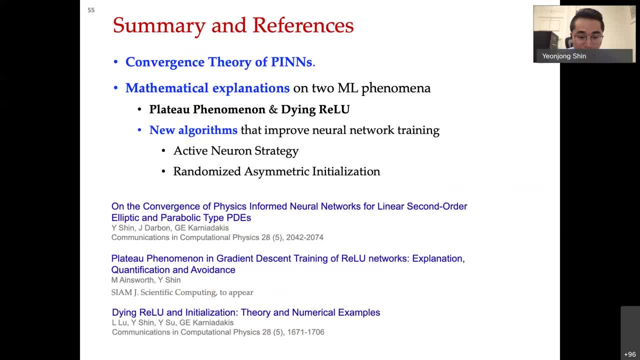 Okay, let me see. If you move your mouse to the top of the shared screen, then there is an option. Ah, okay, There's a chat option. Okay, so that you can have access to. Okay, the question from Lauren. the first question. 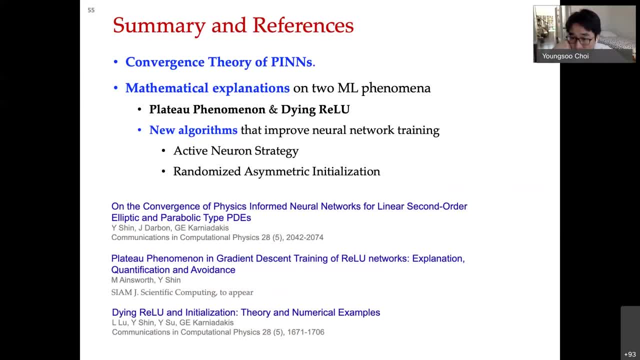 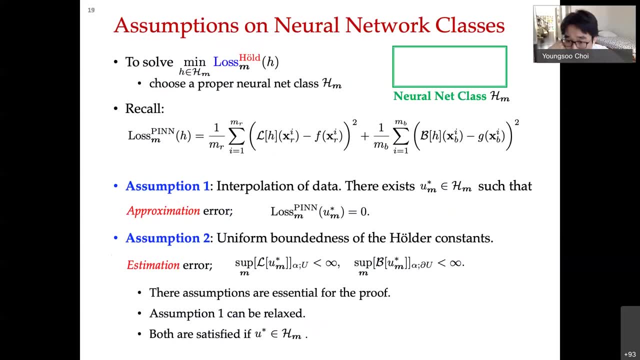 Is regarding slide 19,. for your assumption number one, which is existence of a suitable, well-behaved interpolation function- I'm not sure I understood that correctly. Is the satisfaction of such an assumption likely to be problematic when the data is coming not from the actual PDE but rather from potential individuals? 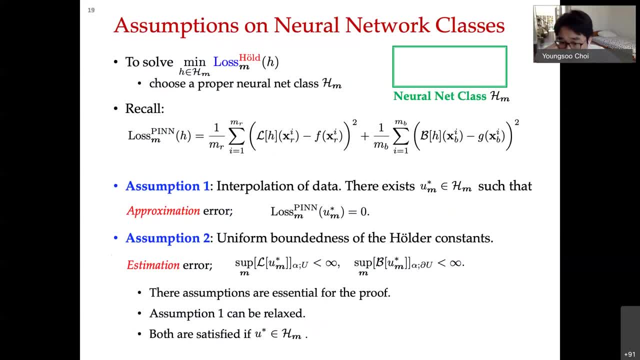 Or is it from potential in noisy experimental data that the PDE is attempting to model? Yeah, actually that's a very good question. So the assumption: don't assume any noisiness of our PDE data So we somehow assume some ideal cases where we don't. 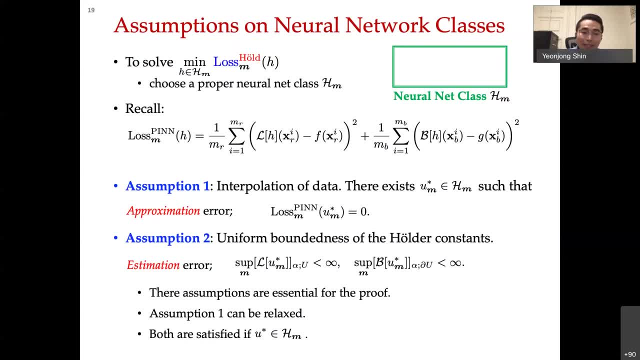 have any noise, but noise can be easily incorporated under certain tweaks. So, as I mentioned here, there are assumption one can be relaxed, So that part actually requires that you don't need to actually exactly interpolate all the data, but there's some allowance you can offer by off, by 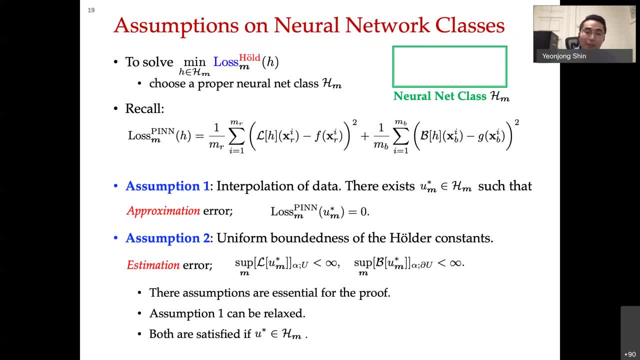 and that is determined by certain rate dependent. But as far as there's some tolerance is satisfied, then you can allow some noisy data. And also, in this setup we are not actually feeding a solution to the PDE rather than the PDE data in the right-hand side. So in most of the cases, 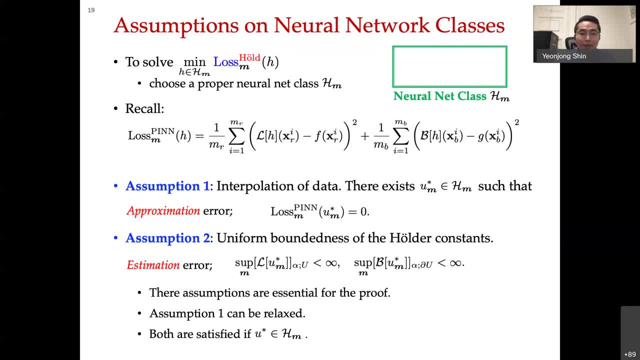 you may know what is your right-hand side or right-hand side f and g, but if the noise level is greater than what it is imposed, then that is a good question. I need to think about a little bit more, But that's a very good question. Yeah, I hope that answers. 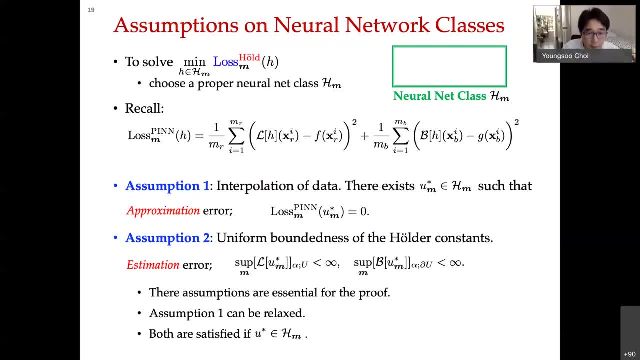 your question. Okay. Thank you, Yeonjong. Okay. Next question is coming from Sampa. He asked: even in finite element method, sometimes boundary condition is not perfectly satisfied, For example, non-conforming meshes. Can we similarly relax the boundary condition? satisfied condition to. 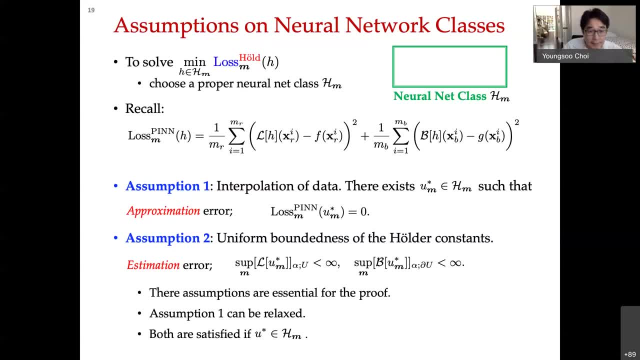 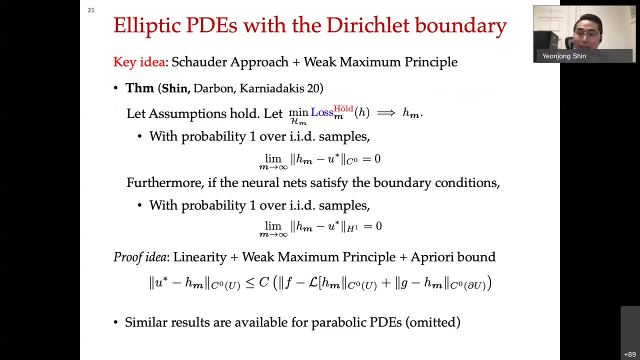 just a converging sequence instead. That's a very good question. Yeah, I think that is possible. That is possible because the – yeah, that's a very good question. Okay, And the next question: Yes, I think there is a possible. Yeah, that is possible. 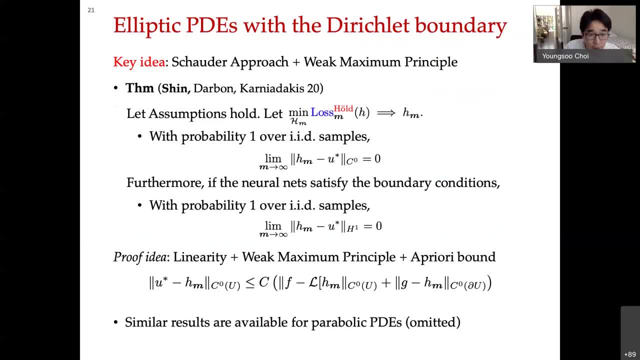 Okay. So next question is from Andrew. He asked for the 2D function approximation example of the Bukin function. did you compare it to any classical interpolation techniques that do not use neuron junction Yes, or danachatariist trouble? Could you explain it a little more"? 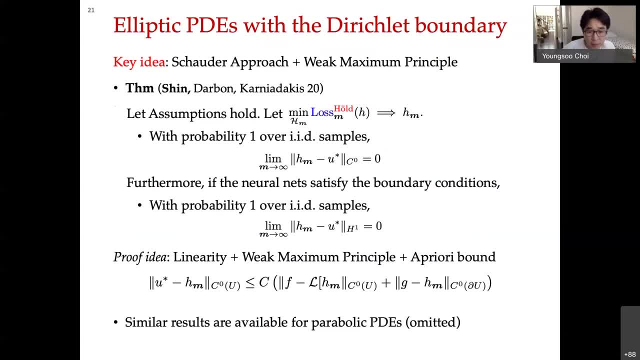 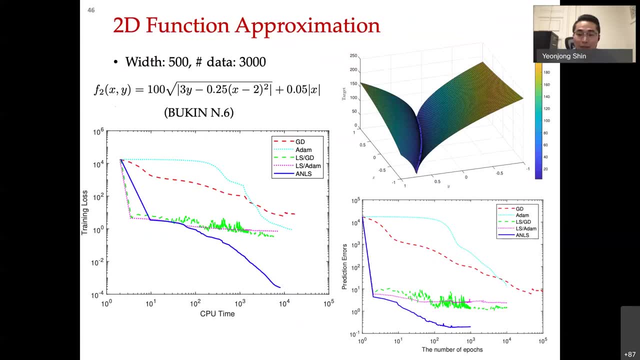 neural networks. they should perform fine in this setting. DR YONGJIN PARKER. Oh, yeah, sure, We didn't test against other classical methods because our focus was to understand how we can improve the neural network training using shallow neural network at the first. So I think the focus is a little bit. 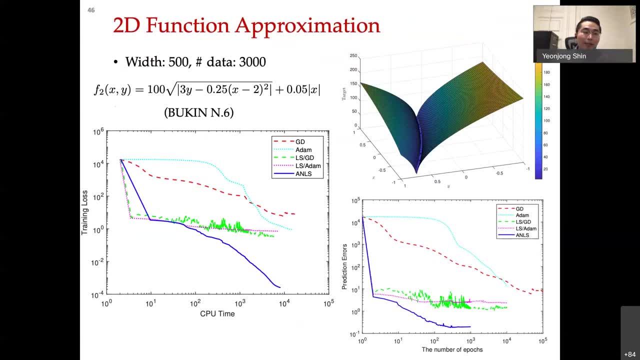 different. So our goal is not approximating to find the best approximation tool that approximates the 2D function, rather than we devised how we can train the shallow neural network compared to existing method. like existing method cannot do, But I do believe that if you use some 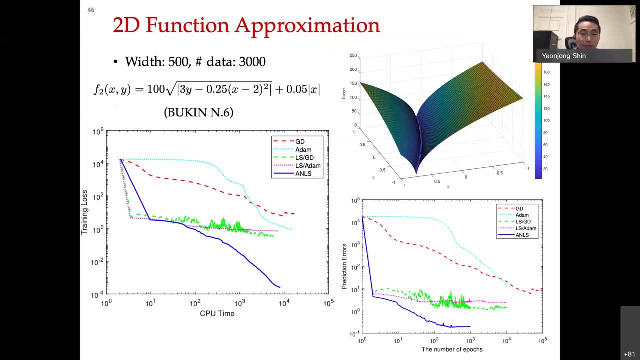 orthogonal polynomial like tensor product or some Fourier basis, would perform well for the task. Yeah, That's also a good question. Yeah, But our main focus was to: okay, let's improve the neural network training, because the neural network training is not very solid at the moment. So, yeah, 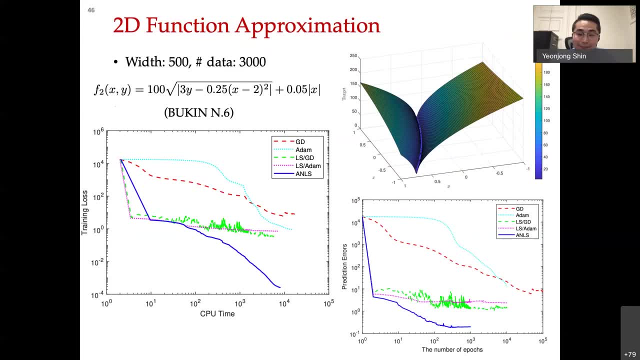 DR YONGJIN PARKER. Okay, Next question is from Sampa. again. He said, just curious, what does the network architecture for the wave equation look like, for example? DR YONGJIN PARKER, It's a very simple neural network. It's a shallow network. 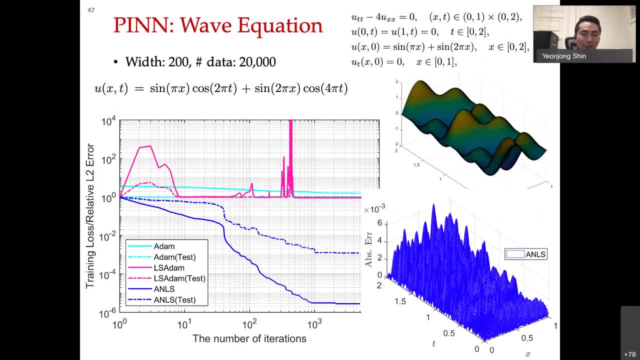 Just DR YONGJIN PARKER, a two-layer with 200.. And we use activation function. is the ReLU power? I forgot what was the order. I think the ReLU cube or fourth power of the ReLU. Yeah, So it is a dense, dense network. 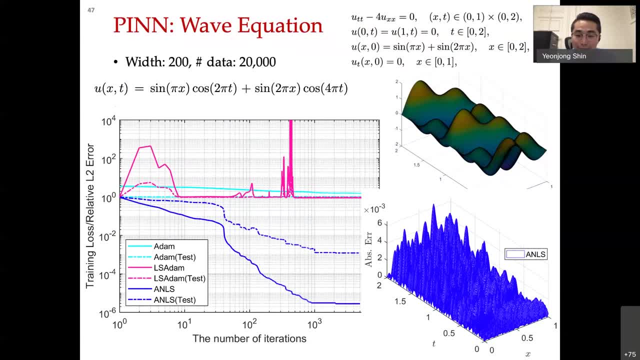 Yeah, DR YONGJIN PARKER. Okay, Next question from Sophia. In any pin cases, did you observe the phenomenon of double descent, DR YONGJIN PARKER, Where a model appears to asymptote, but if you give it enough time and epochs, you will observe another descent in error? 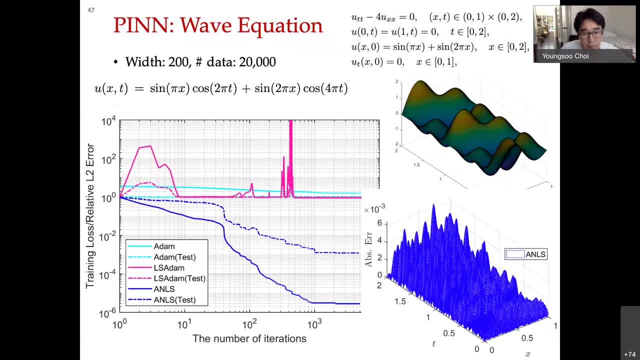 DR YONGJIN PARKER. That's also a very good question. I haven't focusing on the phenomenon of the double descent because double descent is sort of like understood along the way of the training procedure, So that in terms of the getting minimum perspective, I 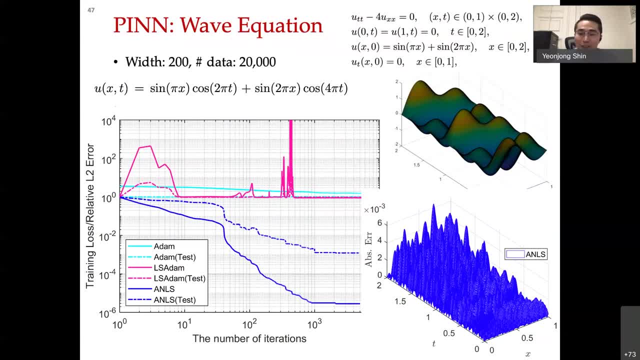 DR YONGJIN PARKER. Yeah, I agree. To get to the question, DR YONGJIN PARKER, yeah, I do, empirically. I do observe some double descent phenomena in training pins, but as you can see in this the specific examples, 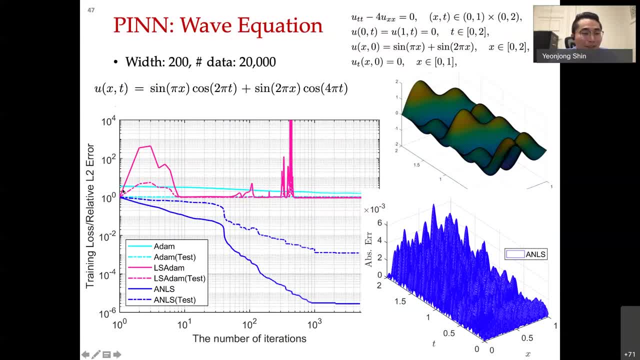 you can treat this as a flight of. I mean double descent. I mean it's an increasing, high and decrease, and also increase, decrease, increase, decrease. You may think of this as a double descent And I'm not sure whether it is also called a double descent, but I do empirically observe. 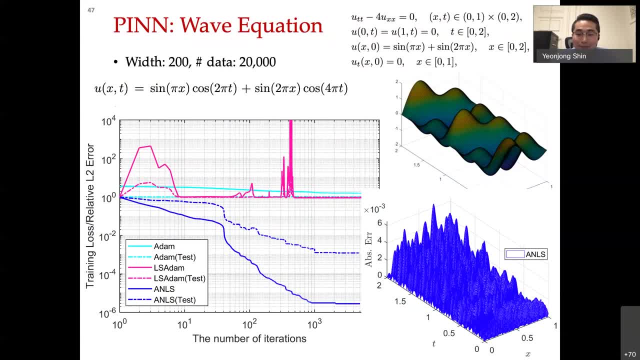 that some double descent. but if you give it enough time and apples, you will observe another descent in error. And that's I'm not quite sure, because I usually run training. maximum 1 million iteration So, but typically 10 K, so I'm not quite sure on that part. 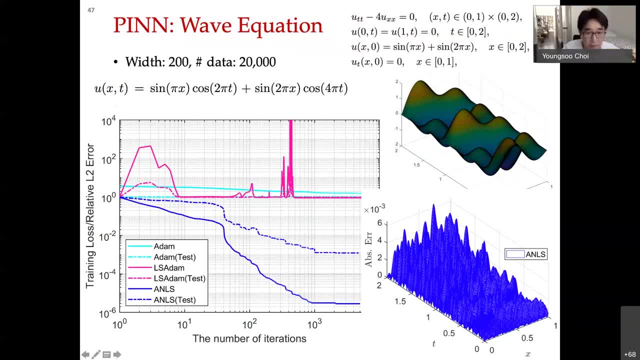 Yeah, That sounds like enough epochs. Yeah, Okay, Okay, So I don't see any more questions from chat room, but you can unmute yourself and ask a question directly. I have a question about the dying probability based on the analysis there. 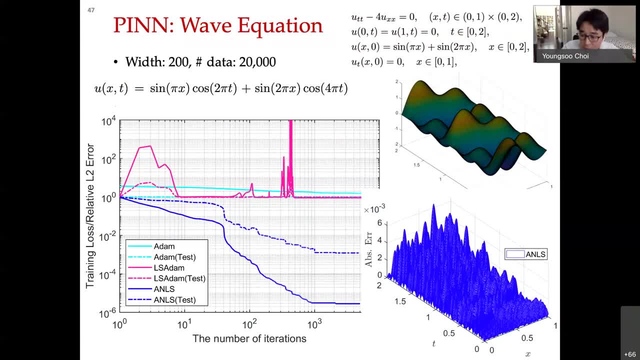 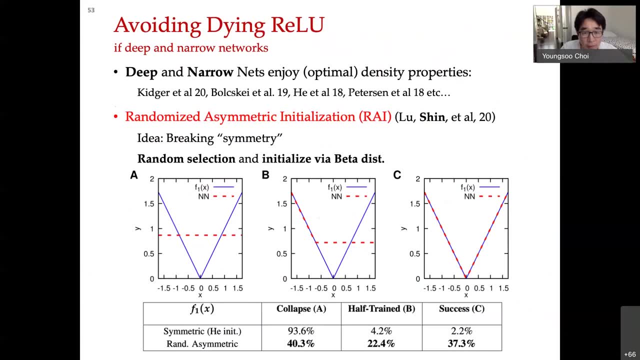 It sounds like it's more favorable. The neural network is The, you know, wide, shallow network than the deep, deep narrow network. Right, But in in practice, you know, the deep narrow network is a lot more popular than the shallow. 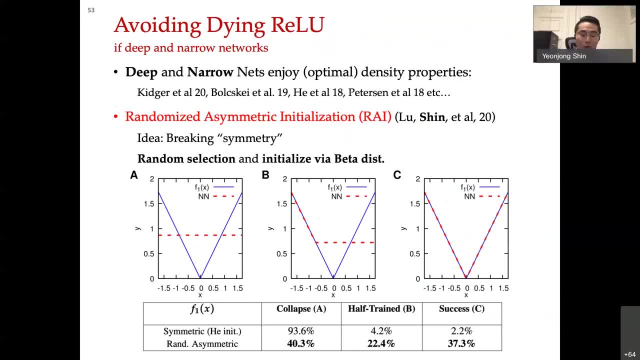 wide network. Yeah, So that that's also a very good question. So I haven't thought about it as a. this is also irrelevant to what I did, but some empirical. my experience is that If you want to express some sort of 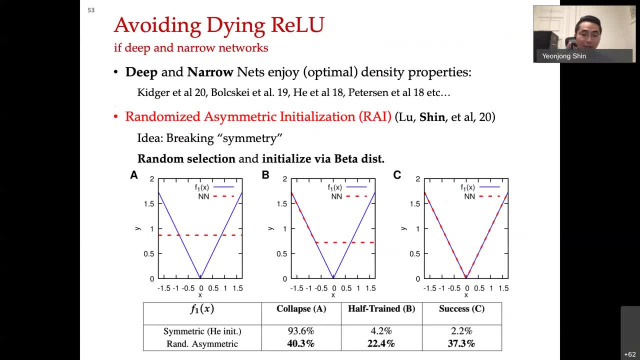 Sharp changing behavior like shock. I would recommend you go with the deep network because that is somehow more oriented to or I would say, more efficient to represent the sharp transition. But if you want to, some smooth behavior, shallow will do the good job. 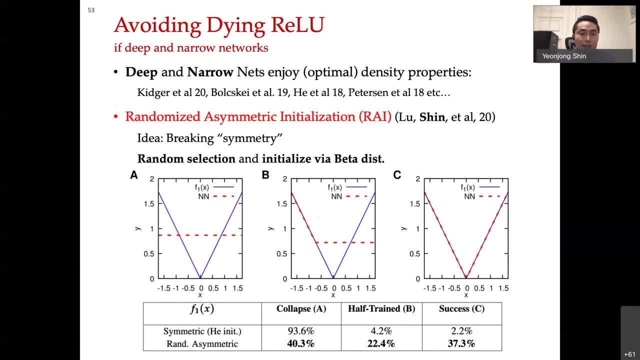 So, and also in practical level, Deep and narrow network. Yeah, I think the deep network sometimes does not work Very well, In multiple reasons, I think. uh, one is the initialization and the other is the uh, the number of the depth quite matter. 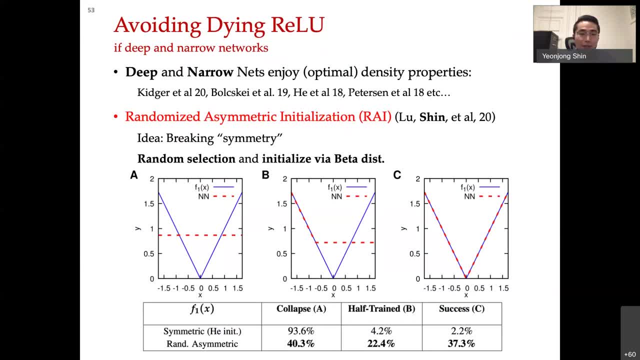 And also the specific architecture view if you use the resonant or some batch. normalization and some other techniques also comes into the play And personally I read a couple of papers that some mean field approach of training, but it is something very far off. 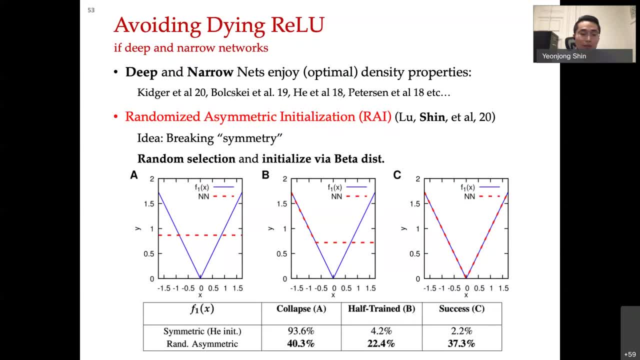 And so there's no one thing that you can do, because you have a very, very, very, very stable neural network. that indicates that super wide neural network can interpolate like almost anything. Yeah, But personally, when I tried, I couldn't quite get the same result. 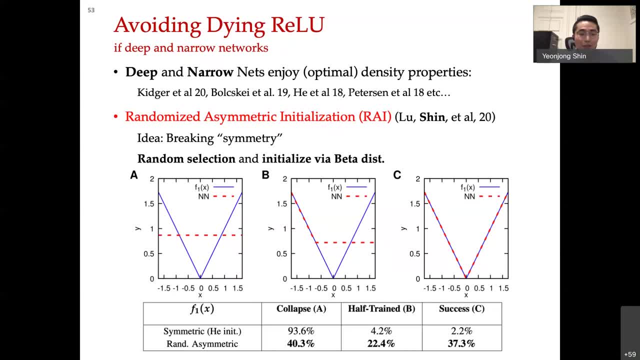 And I think the one of the reason is that theoretical one on the stands that when time goes to infinity or a certain number of iterations, uh, then you will achieve some certain desirable error. But in practical cases what I can do is just a 1 K or 1 million iteration. 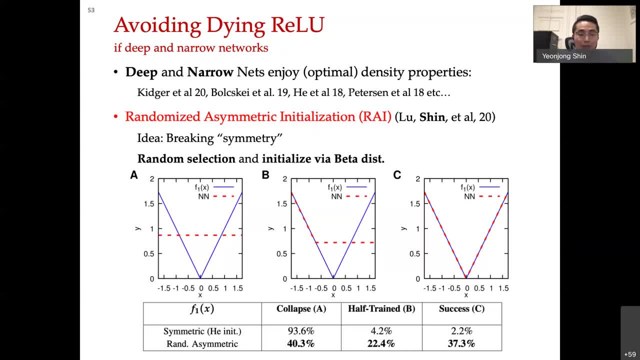 It's a lot easier k or 1 million iteration, so probably that might be one other reason i might see. i hope that answers what you ask. yeah, yeah, okay, um, i don't see any more questions. um, is there any? any? any, any person who wants to ask directly? um, can i, can i ask a question? yeah, yeah, so so you, you showed that a. 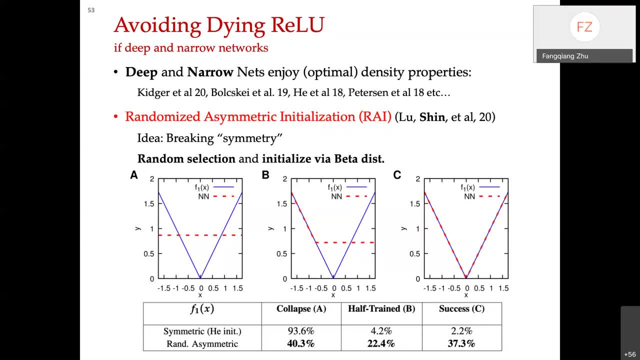 anls method is a very good tool, uh, to solve the- um, fatal problem. um, it must be my fault, i, i didn't some, i somehow didn't catch. what is that method is about, how it differs from the traditional method. can you like briefly remind me about that method? uh, active neutral is the square. yes, oh yeah, so. 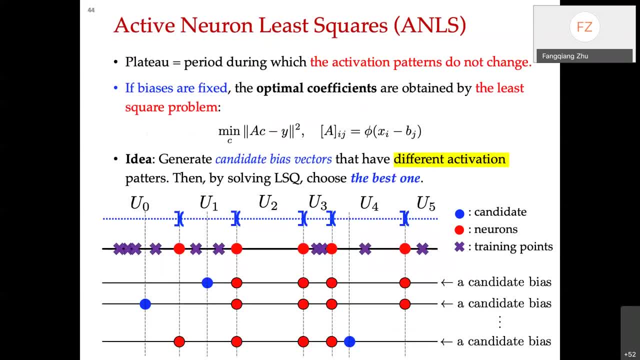 actually i didn't explain it. uh, how, the how it? this method can be extended to the multi-dimensional case, because that is the will upcoming soon. but the main logic is that explicit adjustment of the activation function, activation pattern, because the stagnation occurs when you don't change your activation function. 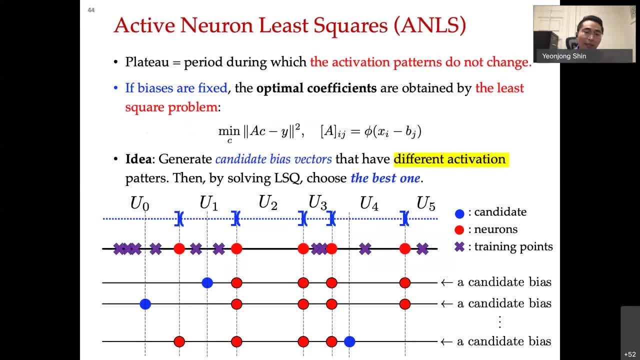 so that we. so what gd takes a long time is that they take a really long time to until they change the new activation function, and then they decay fast again. so our idea is all right, then. since the changing activation function, activation pattern, takes a long time for traditional method, then why now we manually changing it explicitly so? 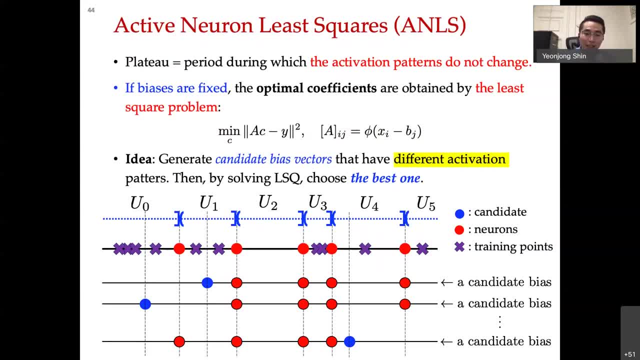 explicit adjustment of activation pattern is the key idea. uh, so, operationally, how, how do you change the activation pattern? ah, so you don't need to access, you need to go over all any um loss function. you can just compare your uh training data and your specific neuron and see how you can change. 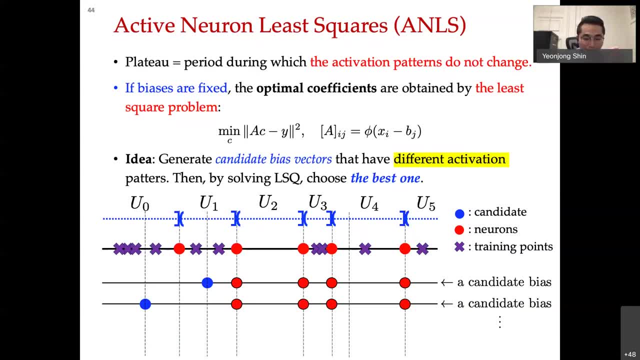 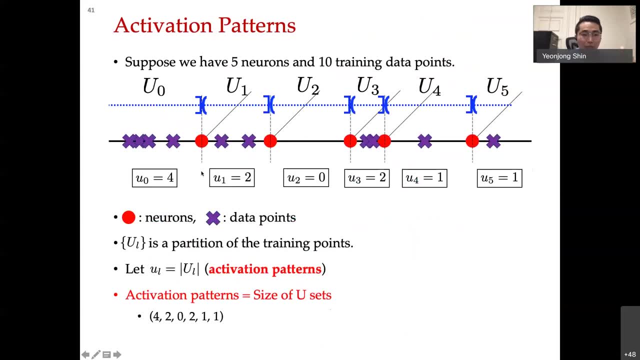 activation fashion locally. so, uh, i think this, uh, so i think this illustrates very well. so suppose this is your current activation pattern, then what you can do is move. move to the left, then this creates a new activation function. right, this creates another activation function, activation pattern. i mean. so this is how we generate. 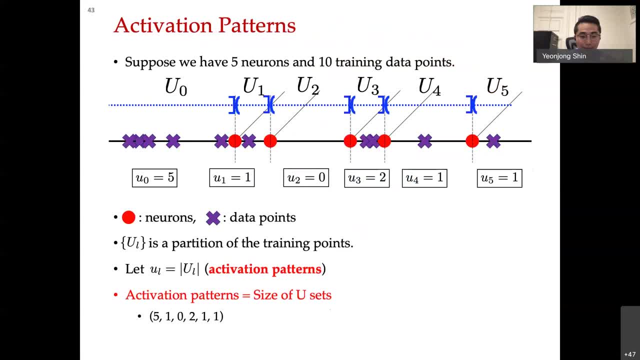 for 1d case. okay, so i'll probably read your paper to for more detail. yeah, thank you. yeah, yeah, so this, this procedure is explained in the public, so it will be to appear on science general of scientific computing. so, uh, yeah, this is what we mean by explicit adjustment of the activation pattern. so 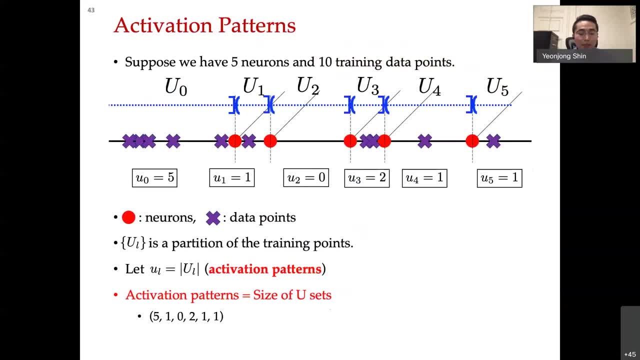 this is the key part: how we can efficiently uh, get a good training result. yeah, that's a very good question. yeah, thank you. yeah, thank you. all right, maybe a little bit more on this question. do you have to manually find the pattern? so i don't. i don't see how clearly i can generate. 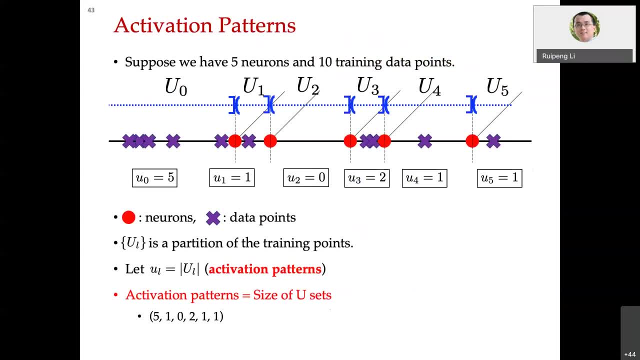 the pattern, the candidate patterns, right. so that's also excellent question. so that's that's why we have a upcoming paper on the how we generalize this, because in 1d case it's left or right, so that is quite easy to see how you can change the activation pattern. 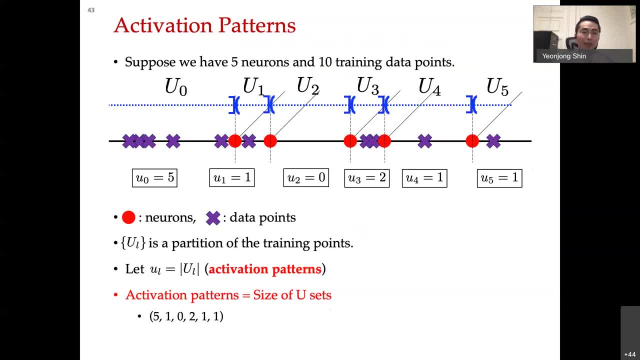 But in our upcoming paper we have a procedure how we can effectively generate the good candidate direction that changed the activation pattern. So it will be upcoming soon. But underlying principle is the same there Because in high-dimensional case the same approach does not apply because there are infinitely many directions you can change. 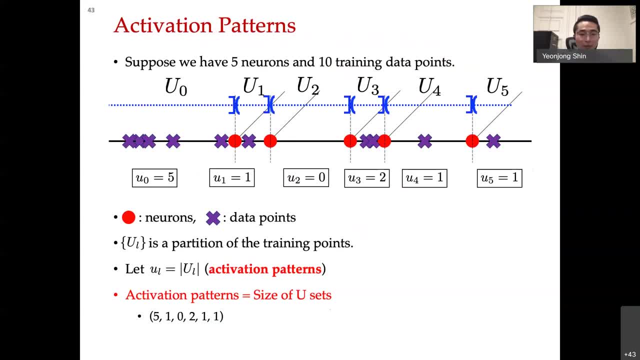 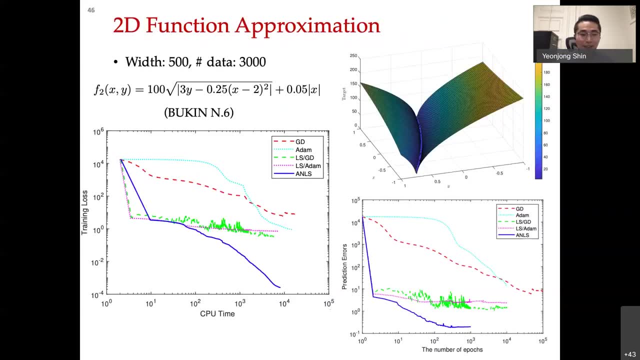 You can generate the activation pattern right. So in general case, we have a way to do that, a more efficient way, so that somehow I slicked into those two rejects in here and here And those rejects will be available soon, probably at the end of this month. 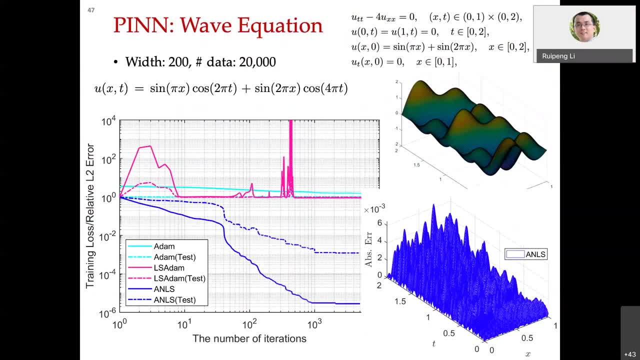 Yeah, that's a very good question. Thank you Great. Is there any other questions? Yeah, I have a question. Okay, Hi Junyo, This is Fan Hi Fan, Hi, Fan Hi Fan. Actually, first I have a question about that wave equation. 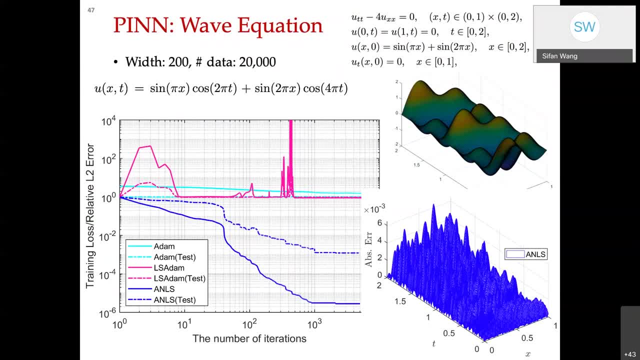 I mean, have you ever tried free features I'm very interested in? is there any connection between the free features and the activation patterns, Because actually free features can do the same thing. but I'm wondering if those activation patterns can explain those phenomena. 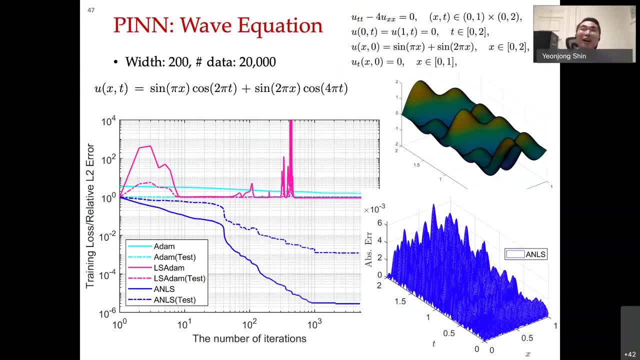 That's an interesting question. I haven't tried how this free feature works. I mean, I think it can be somehow applied. Actually, I'm not sure whether you remember this example. Actually, I borrowed this example from one of your paper, I think. 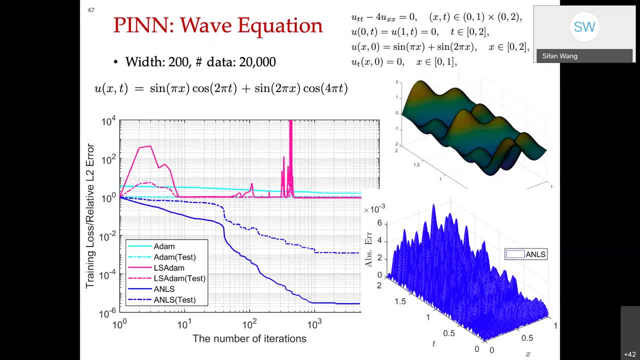 Yeah, I'm very familiar with this example. I had a hard time hearing that. Yeah, actually I haven't thought about it in that direction, but I think it must be related to activation pattern. I think So that by applying the free feature transformation somehow, your input is somehow easily. 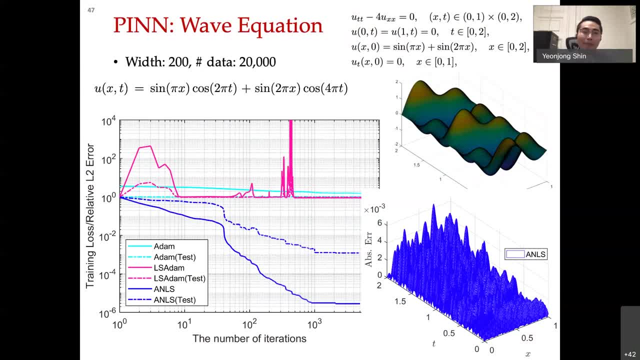 somehow become easy format that can be easily changed the activation pattern in some sense, And it should be the reason that we give us a better result. That's my, just a high-level intuition, But I didn't know the detailed comment on the far of this. 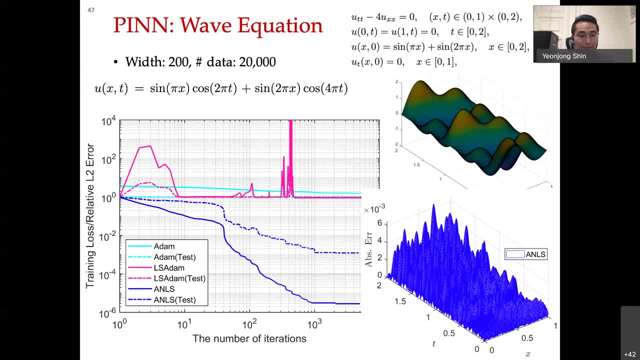 But that's a good question. yeah, I think. Regarding to my second question. So are you interested? Are you interested in that? are you familiar with some theoretical or approximation theory of like deep-on-nets? Yes, I did one work on the deep-on-net approximation. 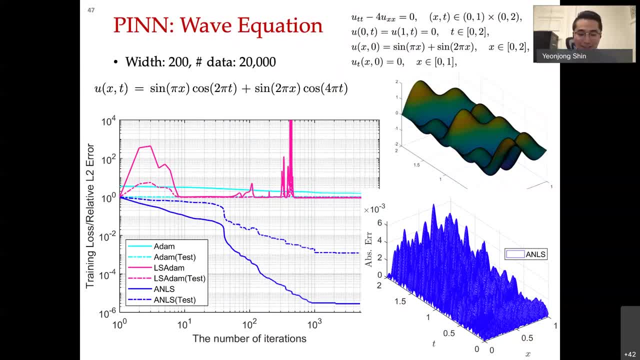 I think this is relevant to the active neural network, right, Yeah, so if this is the case, are you familiar? So are you interested in like deep-on-nets with some physical, basically physics-informed, loss? Yeah, sure, Yeah. 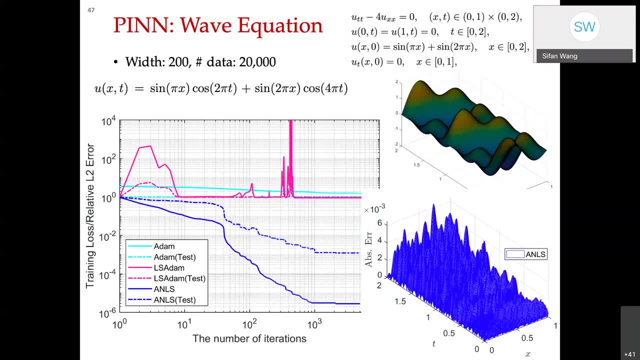 Okay, thank you so much. That's all. Yeah, but I haven't tried the training deep-on-net. but yeah, yeah, thank you. It's a really nice presentation. Thank you so much. Okay, next question from Surabh from chat room. 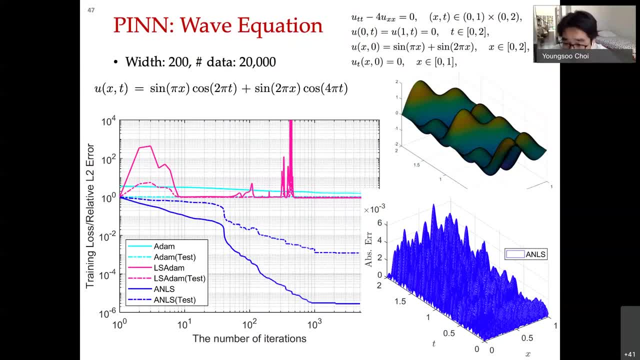 Can the PLATF2 phenomenon be addressed with an adaptive learning rate or gradient-based annealing methods? If so, how do these methods compare with with the performance of the ANLS algorithm? Hmm, adaptive learning rate and gradient-based annealing method. 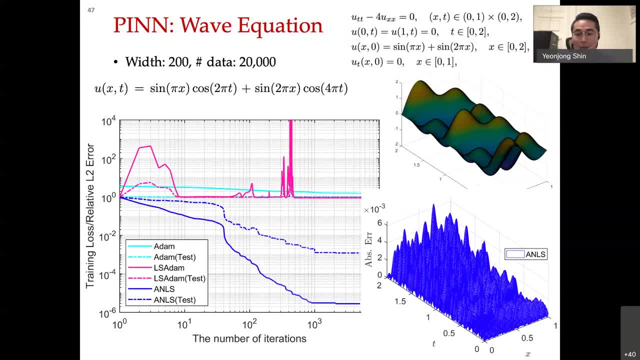 Um, I'm not quite sure how this adaptive learning rate and gradient-based annealing method uh will. I think we follow the similar principle that you just mentioned In our upcoming paper in addressing the multidimensional case, because we're also utilizing the gradient information that suitably change the effectively change the activation pattern. 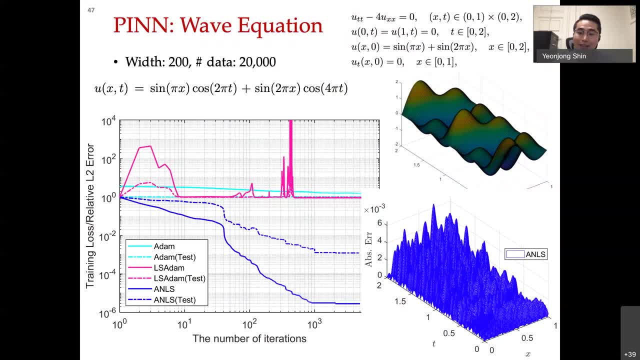 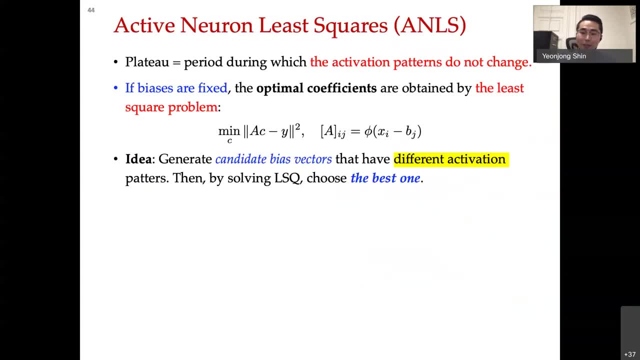 So one great feature of the ANLS algorithm is that it can be used in a variety of ways: gradient-based annealing method. so if you are mentioning adaptive learning rate, is the? i'm not quite sure what exactly adaptive learning rate, but if it is meant to be, 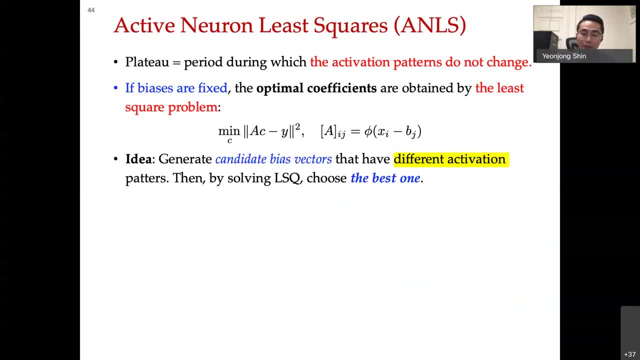 some scheduled learning rate or some other uh learning rate. uh configuration, we haven't really tested, so we just fixed the adam to be a default manner, or in some cases, though, we somehow find tuning the learning rate but constant learning rate. so i hope that answers question, and i'd like to know more about gradient-based annealing method, if there exists. 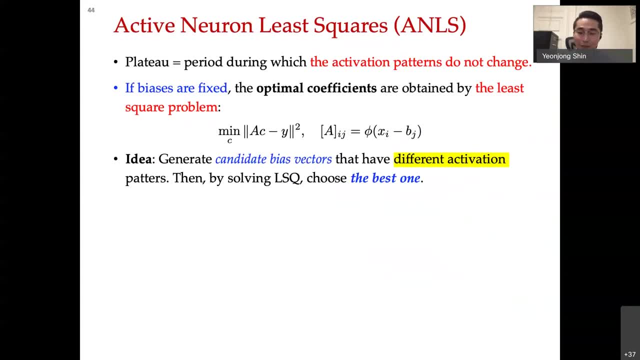 some packages. i can run it to compare. they will be nice. okay, all right, great um. any other questions? um, i guess it's time to wrap up. um, but please do not um, do not reluctant to ask question. if you have no, okay, well, let's thank uh yonjong for the great talk um, i really enjoyed it.